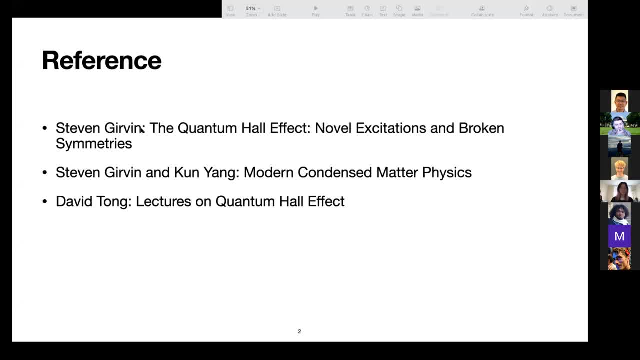 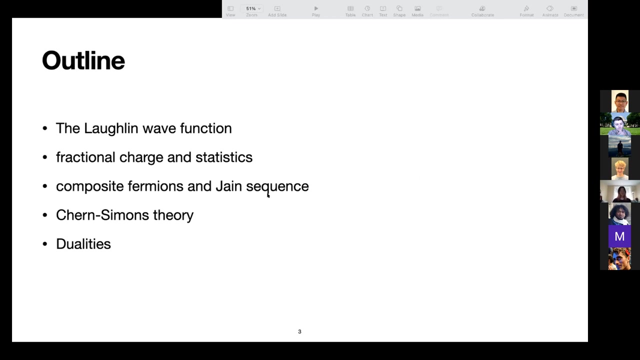 such as the lecture notes by Stephen Gervin and the chapters in this book by Gervin and Young. There are also lecture notes by David Tong which are very good. So today I'll be- this is my outline- So I'll be talking about some basic stuff of fractional quantum Hall and an effective field theory, which is a transcendence theory. 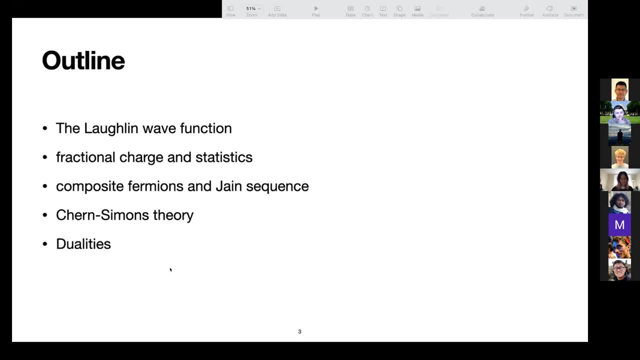 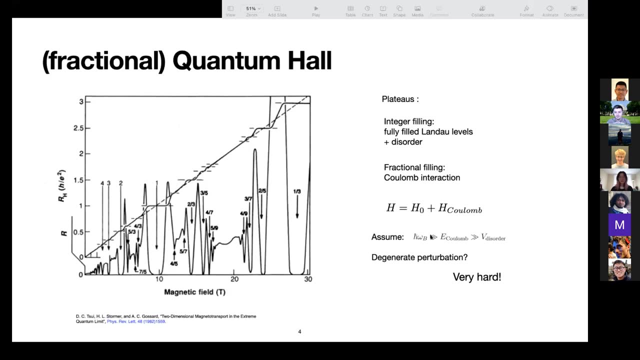 And if I have time, I'll talk about dualities and to make contact with previous journal club topic by Robert. So let's get started. So this is the famous Hall measurement. So, as we can see, there are some plateaus in Hall conductance at integer fillings, which are called integer quantum Hall effect. 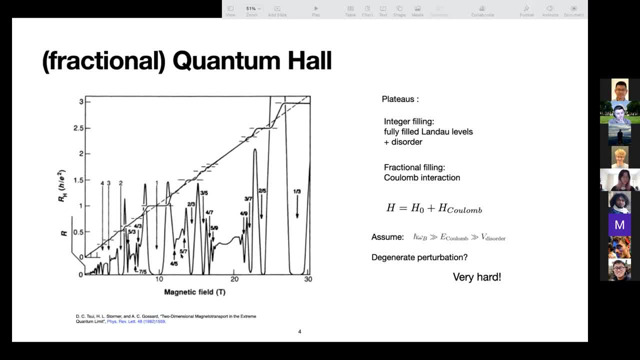 And also as some fractional fillings. So we are all familiar with integer quantum Hall. Basically it can be explained by a fully filled London levels of to the electrons, to the electron gas and magnetic field and plus some disorder which caused the plateau. 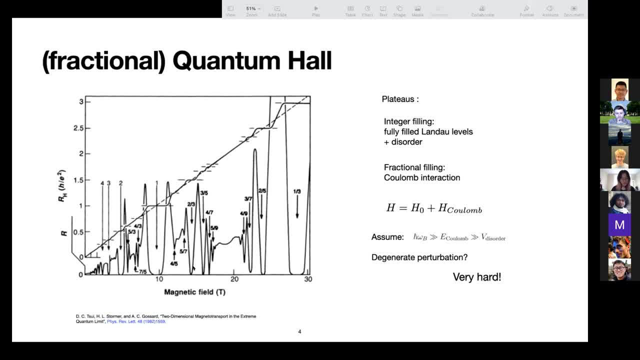 But So for fractional feeling it's a little bit weird Because if we consider, Consider a partially filled London level is since There's no, I mean, if we do not include any electron, electron interaction, there's no way we can get an income. incompressible state. 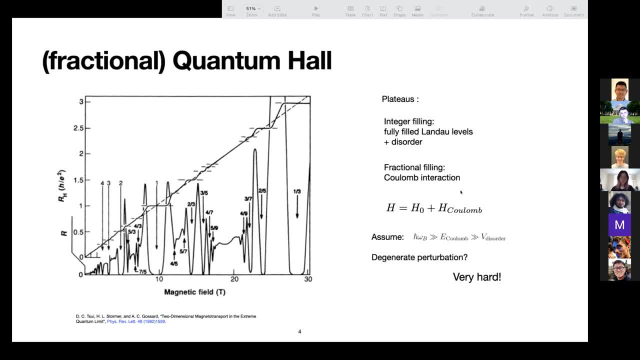 So that means Coulomb interaction must be very crucial in this fractional quantum Hall context. So And during there, So for the rest of my talk, I'll assume this hierarchy of energy skills, which is disorder, Much less than the Coulomb interaction, much less than the London level, splitting. 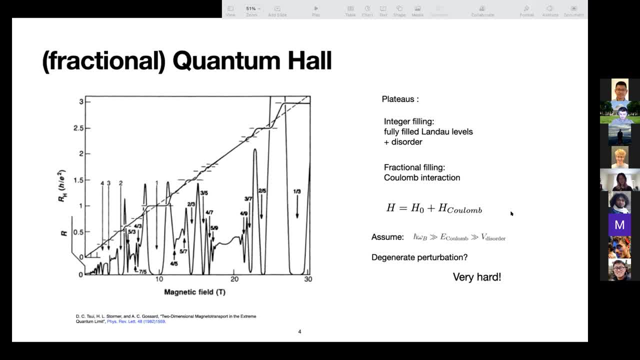 That will allow us to work with the projected states living in, say, lowest London level or a few London levels and ignore the London level makes sense. So with that, the Hamiltonian we're considering is basically basically contains two terms. One is: 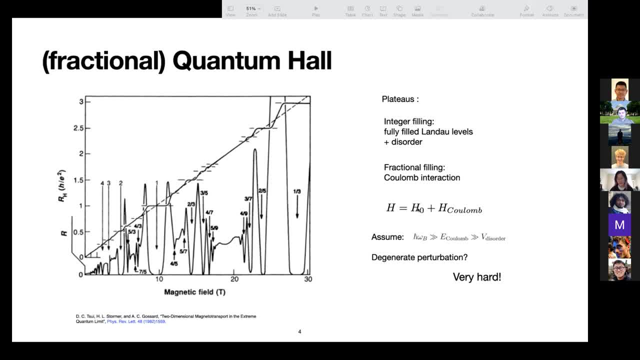 Some Electron gas couple to External magnetic field. We all know how to solve that. it will give us London levels. The other one is a Coulomb interaction. So We are taught to do perturbation theory During our like in the grad courses. but notice that if we have a fractional feeling. 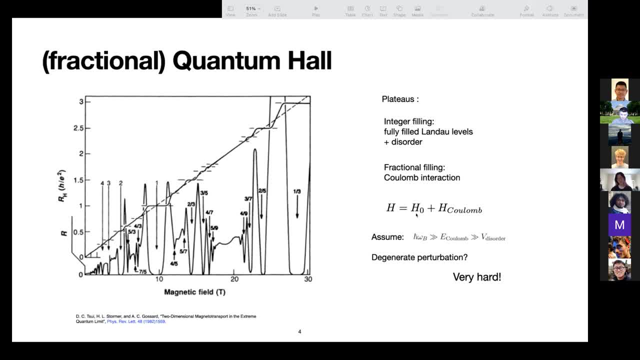 The, the, the grass, the degeneracy of this, the grassroots of H naught, Their degeneracy is huge, So it's a very hard problem to do the general perturbation, But So, So lovely, made a very bold move. 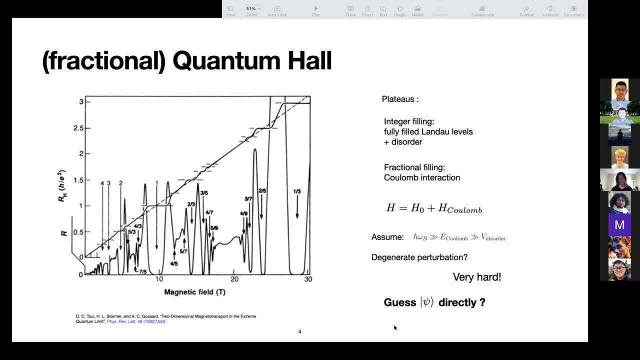 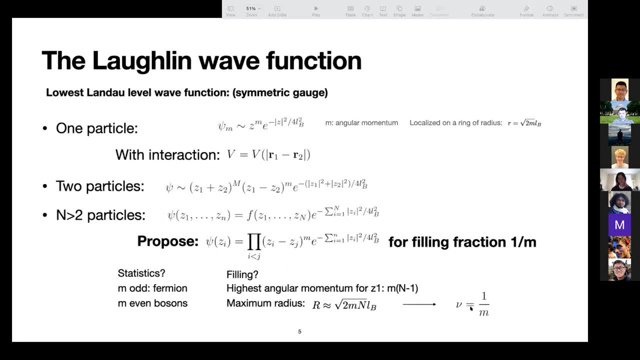 He's like: how about just guess The way function directly? I mean, after all, that's what we want, So yeah, so, So let me introduce the guests way function, which is the lawfully way function. and Yeah, let me just motivate. 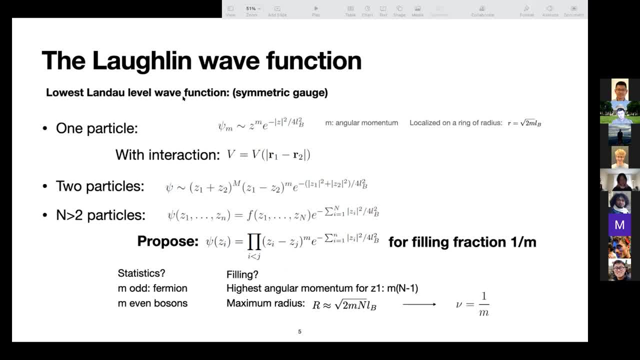 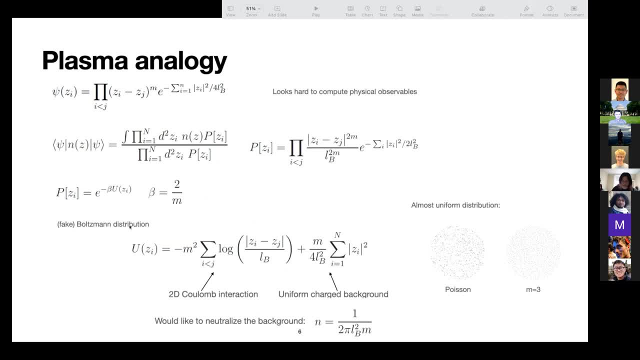 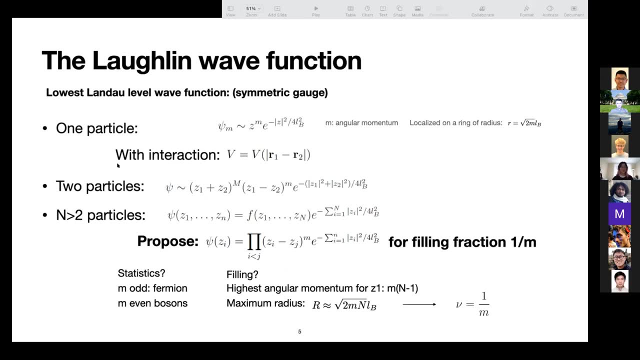 How? Let me just motivate This, Sorry, Yeah, let me just give you some motivation. So for If you, if we consider a single particle state, The wave, and assume assuming symmetric gauge, way for the way, fashion for lowest London level is just some hollow morphic function, times and exponential. 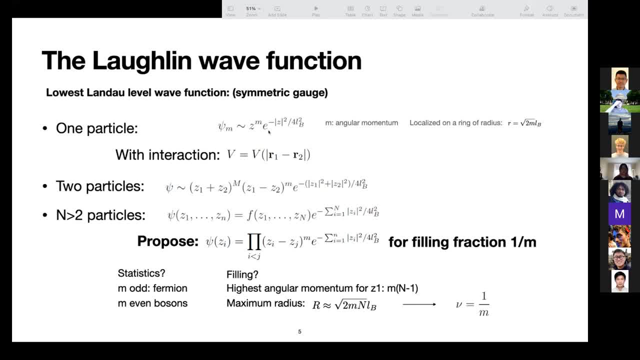 Decay Component. So the The power here And it's actually actually labels angular momentum And this way fashion actually localized on the ring of radius, Which is square roots of, proportional to the square root of M, and times the magnetic lens. So 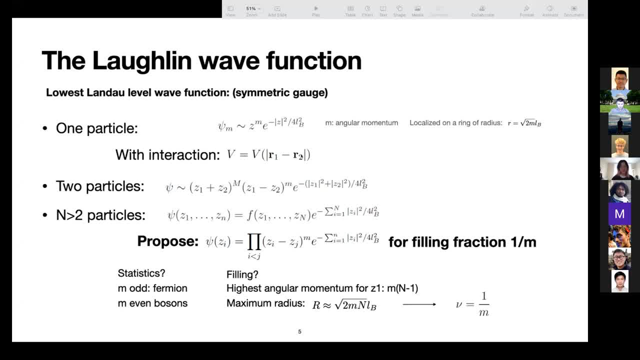 With, With the interaction between two particles, we can consider the grass day wave function of the two particle states. Hmm, Luckily, if we Decompose the coordinates into a relative Relative displacement, and there and We, we and solving the Hamiltonia. 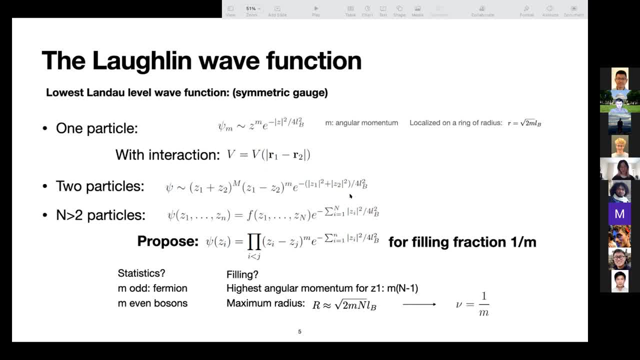 With this interaction we can see the two particles There is actually in this form. So In general it's, I mean, for N equals two particles. It's impossible to solve this Hamiltonia and write down the ground state wave function, but we know that it should be of this generic form with the hollow morphic function that. 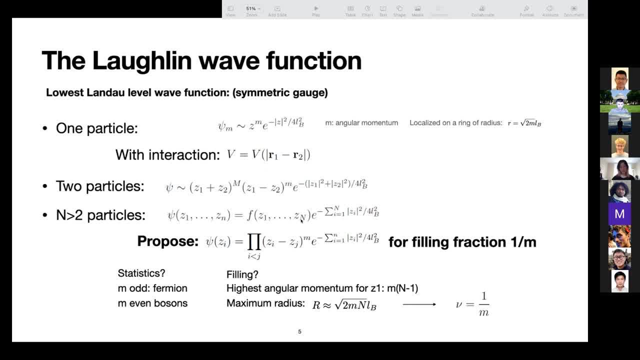 That depends on c one to the end, if we have n particles and they should be an anti symmetric, as we're considering. for me on this, for me on the existence, So motivated by this, to particle function, This c one minus c two to the end seem to be very cute. So I mean we can. 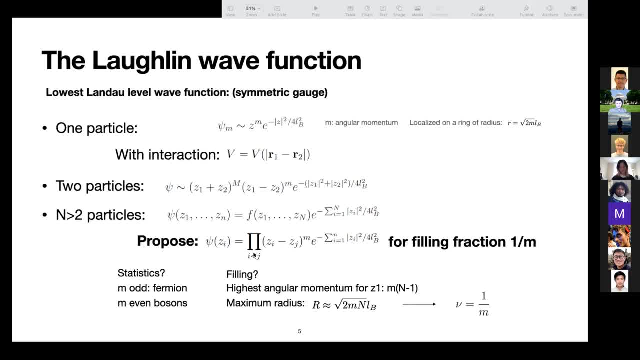 So Laughlin proposed this kind of wave function For a filling fraction, One over m Fractional quantum whole states. Hmm, Okay, so Let's just forget about the Hamiltonia for one second. for one second and to study this wave function directly. 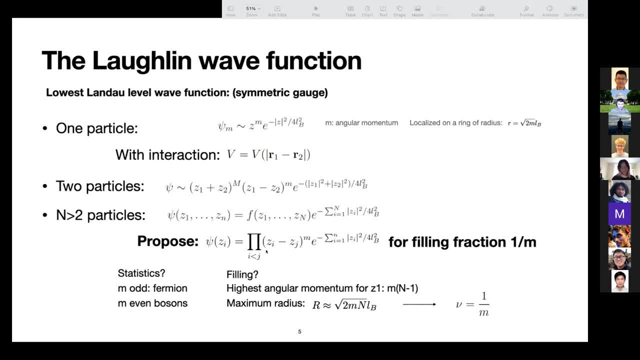 Hmm, So indeed, if m is odd, If m is odd this: This wave function describes the Fermionic systems. If m is even, that's a wave function for bosonic system. But how about the feeling? How do we know the feeling fraction as well over m? 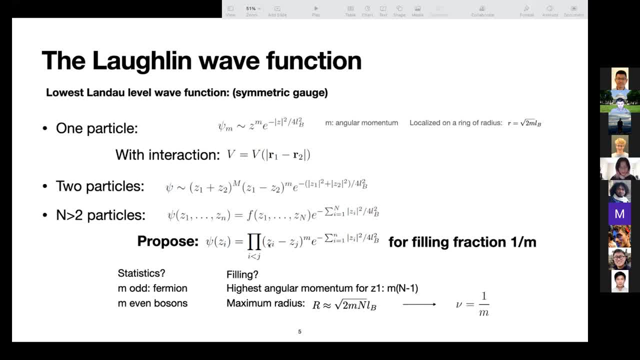 So note, Notice that the highest angular momentum for, say, c one Is m times n minus one, where n is the total particle number. As we said before this, This power is actually, is actually related to the Ring of the radius, where the part, where the part, where, where the 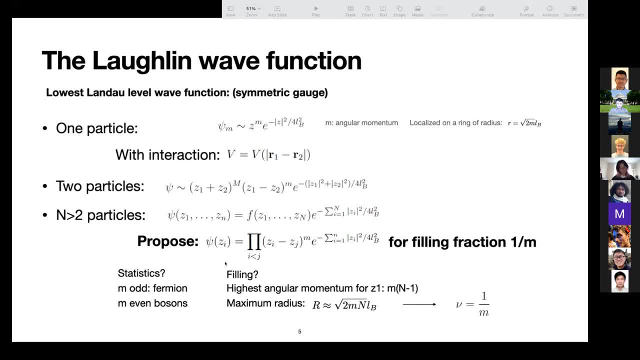 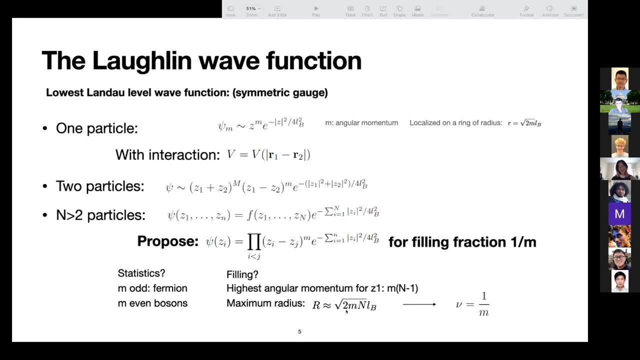 It's proportional to, I mean as thermodynamic limit, where n goes to infinity. we saw this minus one, and this is the maximum radius for the whole droplet. And there are, and we have, n particles In total. so In total, so we can compute the feeling fraction of it it will give. it will simply give us one over m. 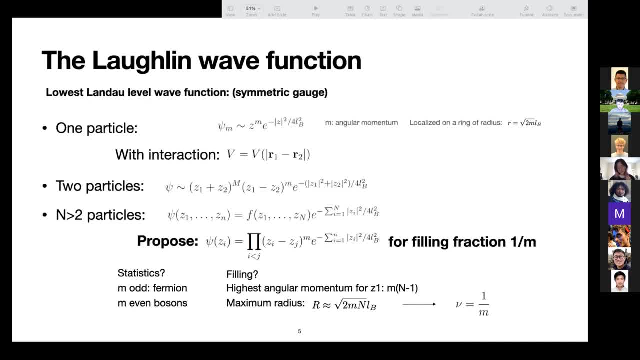 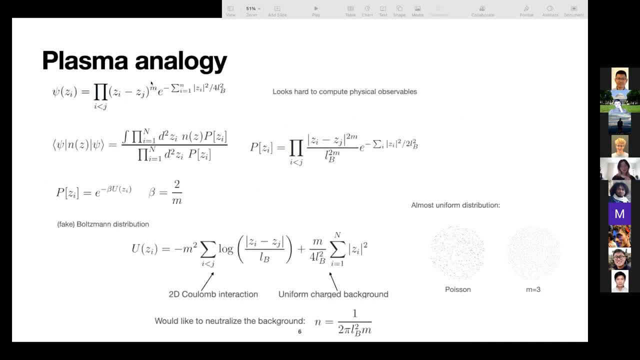 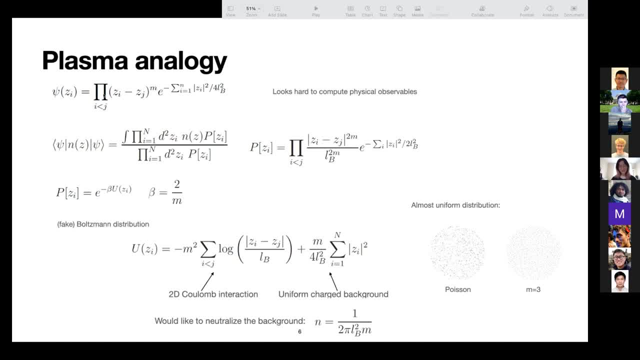 Gage-dependent. here You're saying why the expectation value of n in that particular psi is independent of the formula, Because our gauge transformations aren't acting as phases on psi or anything. I'm just thinking to myself that the form for the wave functions would look completely different in that. 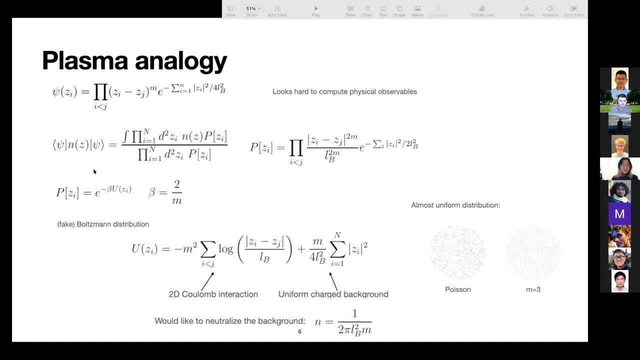 Yeah, in a different gauge, right Yeah, but n here is just some. I mean it's just a delta function. I mean this is a physical observable, It shouldn't depend. It shouldn't depend on any gauge choice. 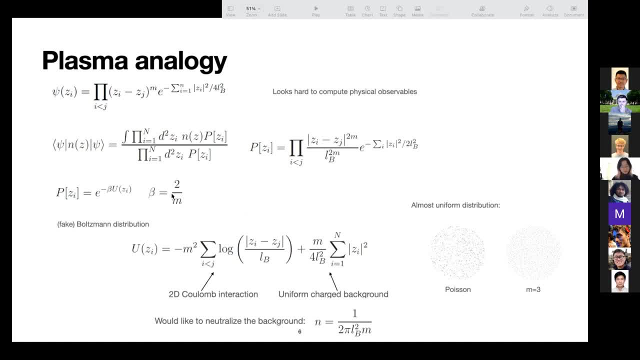 Yeah, and this plasma analogy, just it's a, I mean it's an intuitive way to see how this to I mean to have an intuition for the property of the wave function. I mean it's not, there's no, actually. 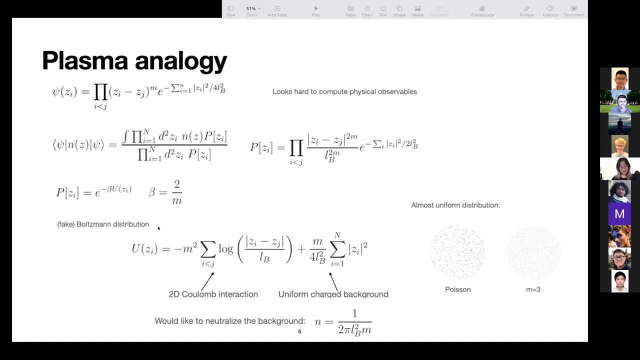 there's not actually a temperature or something, Right? OK, so even though the whole wave function is localized in an exponentially localized in a droplet, the claim is that the density is still uniform. Yeah, yeah, the density is almost uniform. 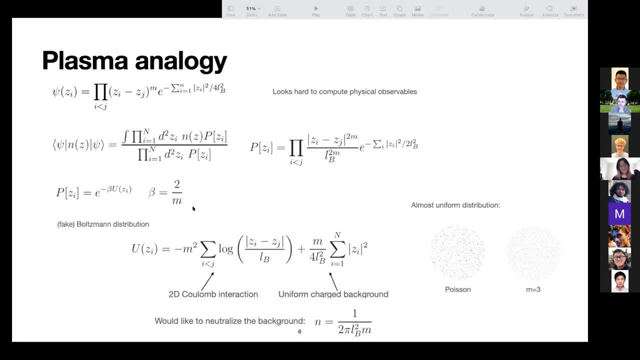 But isn't that weird that, since psi only has like is exponentially, is only supported on a compact region, OK, well, whatever, OK, This is just writing for the Yeah, that's, I mean, that's, I agree. 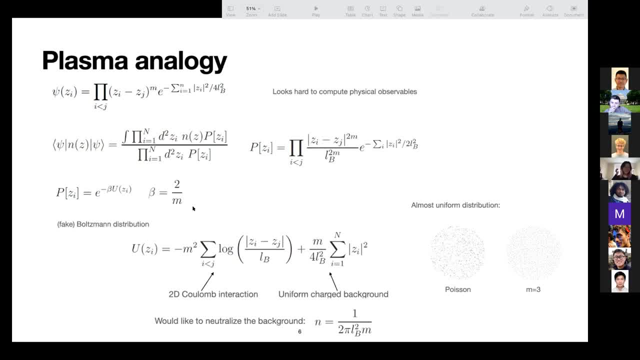 that's very counterintuitive, Yeah, but if you think of it in this plasma way, it seems it also seems a natural conclusion. I mean it's not. I mean it's not at all obvious from the form of the wave function. 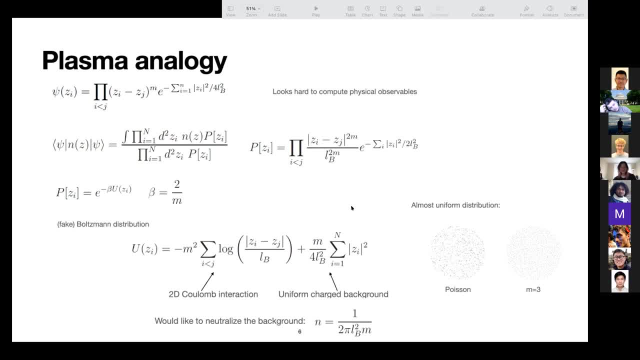 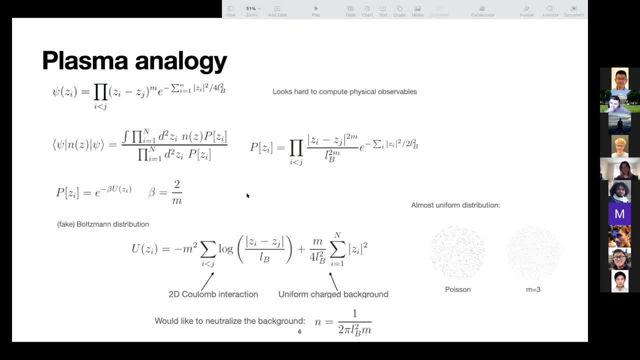 and yeah, so one may worry about whether this guy, whether if this weather these charge, will froze stuff like that. Yeah, but so it? what do people did numeric on these stuff and find that for m, say less than 70 or something, there's this like oz is 10M3. 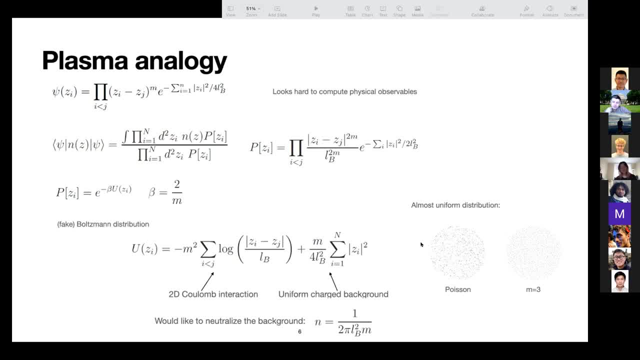 That's a huge lot and it does not expect for enemies of m to respond to the additional energy 내. this uniform distribution picture actually works pretty well. Yeah, OK, Oh, go ahead. Sorry, any other questions? No, I was just saying maybe I'm being stupid here. 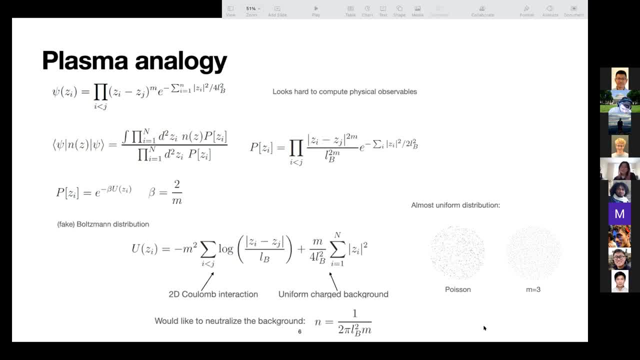 but it being localized to a ring. that was with the wave function, right. So if you were looking for some place for gauge dependence to rear its ugly head, I mean that's probably where I would look Once you look at the charge density here. 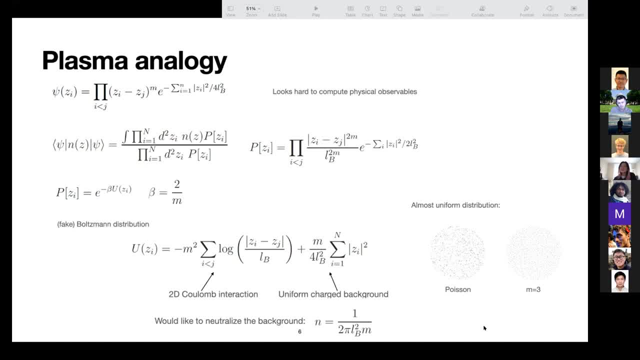 that's where you're applying a plasma analogy, right? Yeah, Right. so I would trust the plasma analogy more than the wave function being localized on that ring, at least when I'm thinking about gauge dependence. Anyway, sorry, unnecessary comment. 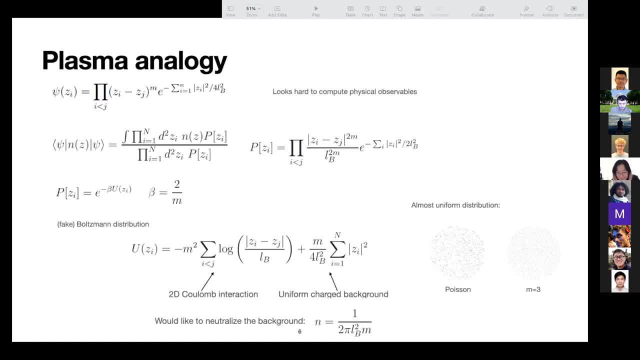 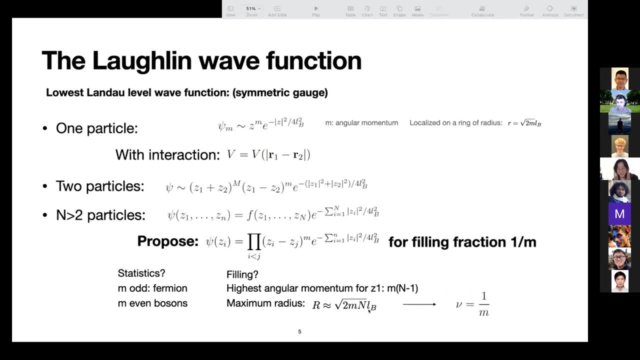 Yeah, yeah, Oh sorry, Right, right Here in the previous slide I just gave a very hand-wavy argument, and it's actually only for one single particle It's. I mean, after all, we're dealing with this. 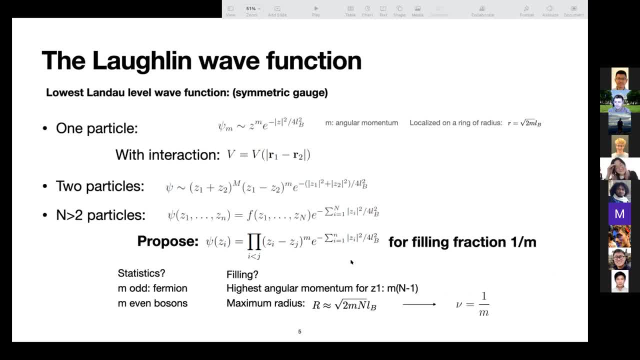 antibody stuff. If I send magnitude of z to be very, very large in the thermodynamic limit or something, it still looks like psi goes to 0. Too fast for it to be able to provide. Yeah, A uniform. Well, anyway, OK. 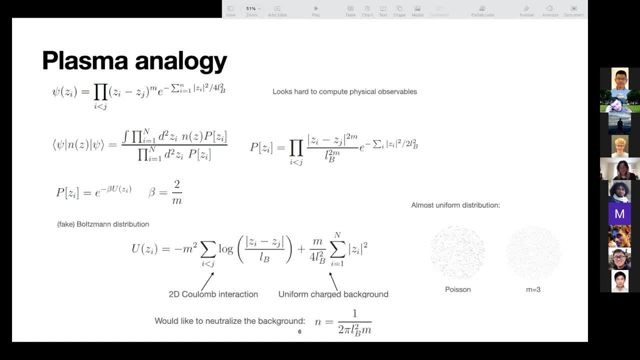 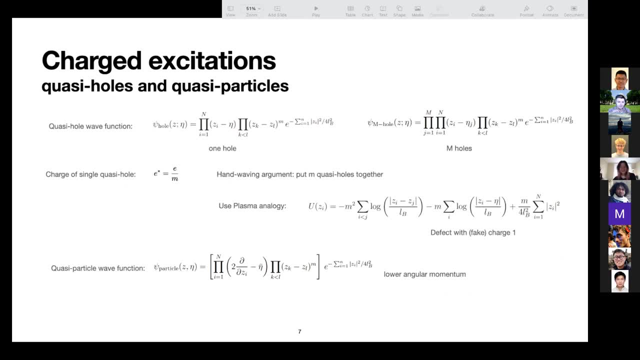 OK, yeah, Right. so far we've only talked about ground states. So let's consider what kind of excitations we can have, So we'll talk. We'll be talking about charge excitations first. So that means we are talking about quasi-wholes. 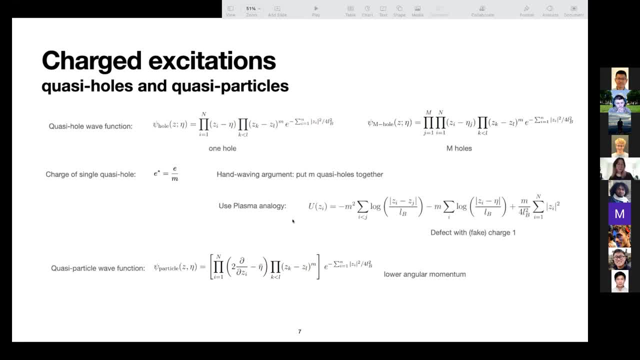 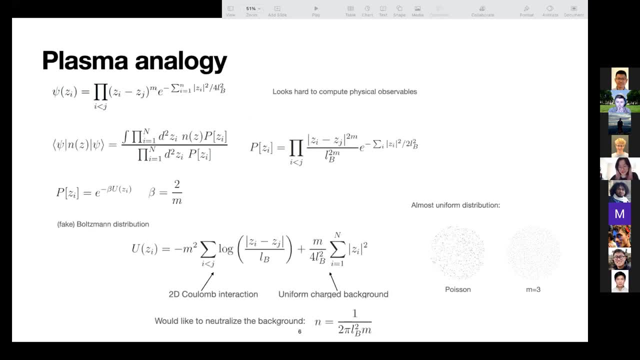 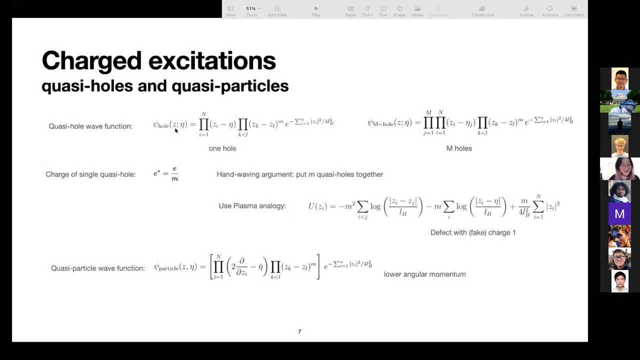 and the quasi-particles. So I mean so in the spirit of guessing wave function, we can just guess the quasi-whole wave function. So yeah, OK, OK, OK, OK, OK, So yeah. so people propose this guy. 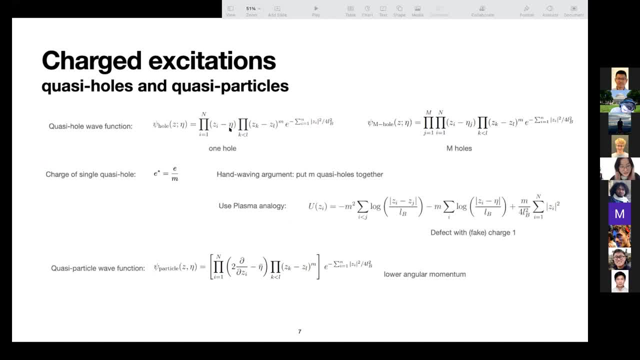 to be a wave function of one whole at position eta. So let's see if this is, I mean if this makes sense. So if I have one whole at position eta, I mean this wave function does have OK. 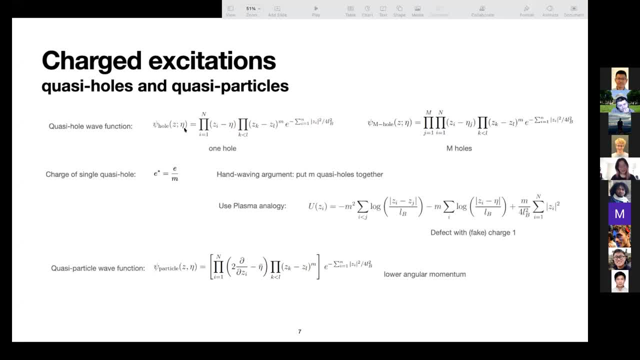 OK, OK, OK, so the wave function does have vanishing amplitude when Z approaching eta. So it looks fine, And we can also try to put m wholes at position eta 1 to eta m. So yeah, this seems to be legitimate. 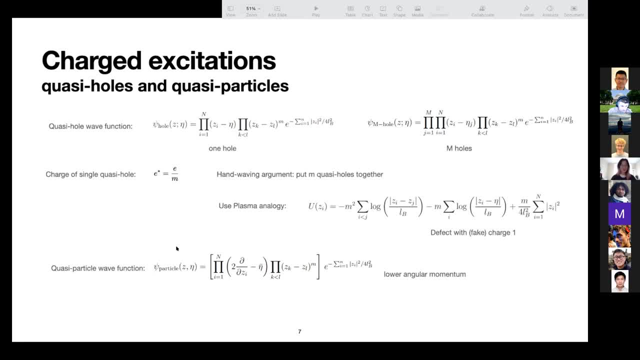 So let's see of a single quasi whole. surprisingly the charge is actually one over m. okay, so i can one hand waving argument is that if i put m cause i hold together and they all at a position eta, then this guy will just be c minus eta to the power of m it. 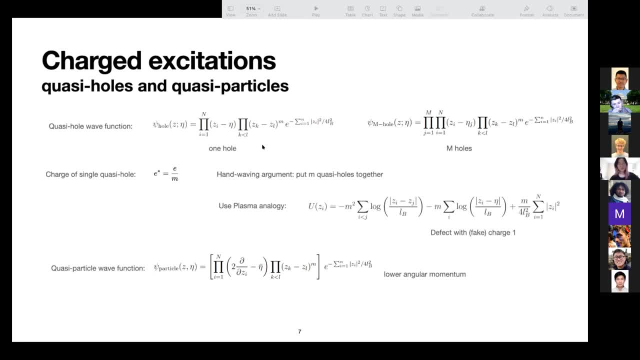 looks like the uh lovely wave function we get before, but so with eta fixed instead of instead of varying. so that means that means we fix one, one electron in our system. so yeah, so that means if we put m whole together, we get an electron. yeah, that means the, the quasi whole, actually has a charge one over m. 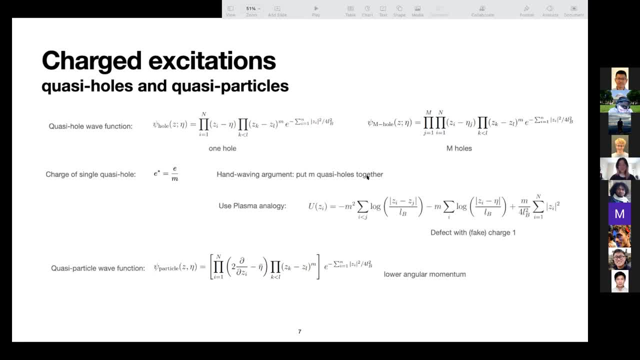 yeah, this may not look very convincing, but so again, we can use the plasma analogy we just learned and write the fake potential, which looks like this guy. so for this one whole function, one whole wave function, we get a additional term which looks like this: it's uh. 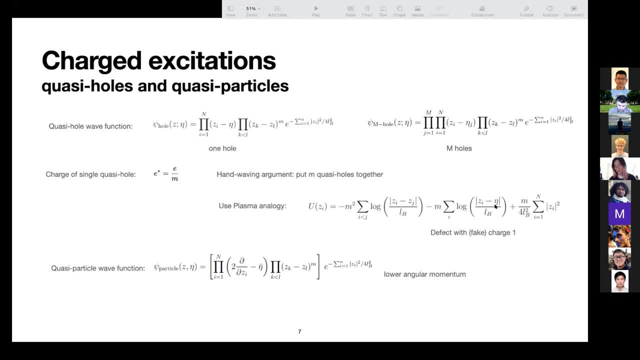 it's a defect with uh charge one. so, right, as we said before, the uh whole purpose of this plasma is want to be neutral. so if i have uh, if i have a defect with charge one, then then all the uh particles will want to, uh, want to be, uh want to come to this, want to screen this fake charge. but uh, notice that uh in this. 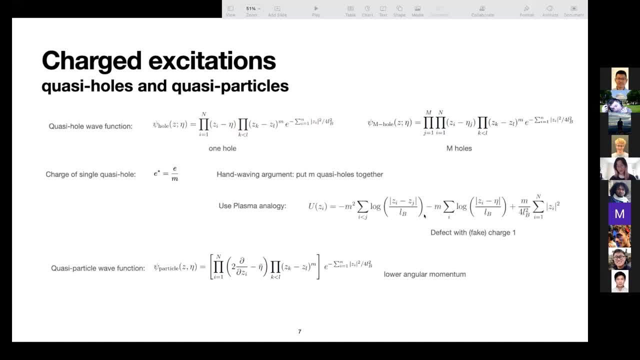 plasma analogy. at the the charge of the particle is actually m, so i only need a 1 over m of the charge density. so but uh, yeah, but the yeah, but the particle actually have has physical charge e. so that means the uh, that means the charge of the quasi whole is 1 over m times the physical charge. 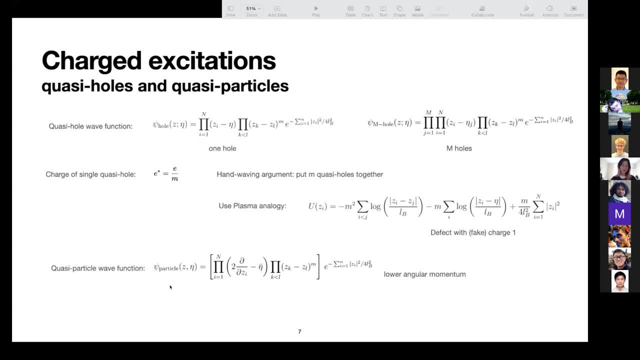 so, uh, we can also consider a quasi particle wave function. one way to consider a quasi particle wave function is that: so notice that in the quasi whole wave function, we want to raise the power of angular momentum, uh, such that, uh, the whole, the quantum, whole, droplets will be larger, but we still have. 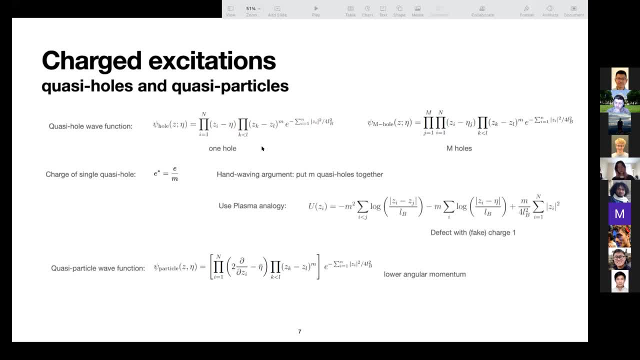 n particles. so it will be uh, so effectively it will introduce whole. if we want to introduce particle, that means we want to lower the angular momentum. so, um, one way to do that is, of course, we can determine the angular momentum of the particle. so we can determine the angular momentum. 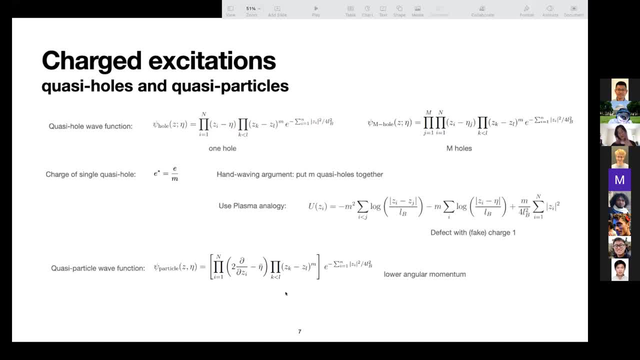 and we can also uh divide the n and the quantum whole itself in the angular momentum, so to say. we can also uh divide this guy by itself once, but then it's problematic because it will introduce a singularity. yeah, but, yeah, but we can also uh multiply. multiply this guy by 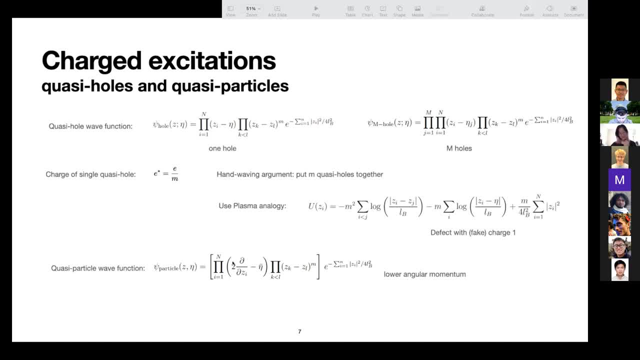 z-bar, that will also lower the angular momentum. but z-bar is not uh wave function. So people did some projection to get this form of quasi-particle wave function. I mean, it looks very hard to deal with and yeah, and indeed I'm not going to talk about. 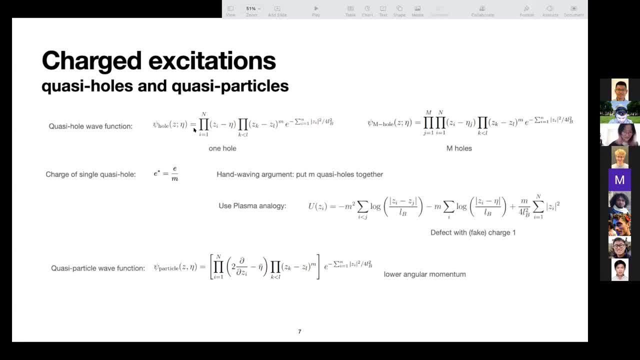 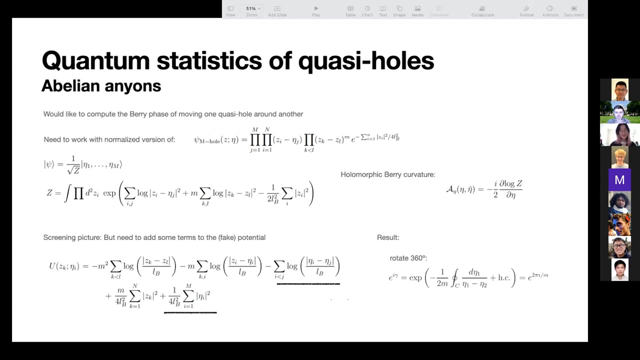 this wave function anymore. I'll be dealing with the quasi-whole wave functions. So yeah, so I told you that the charge of a single quasi-whole is one over m, but how about the quantum statistics of these guys? So that means, if I exchange two quasi-wholes, what will I get? 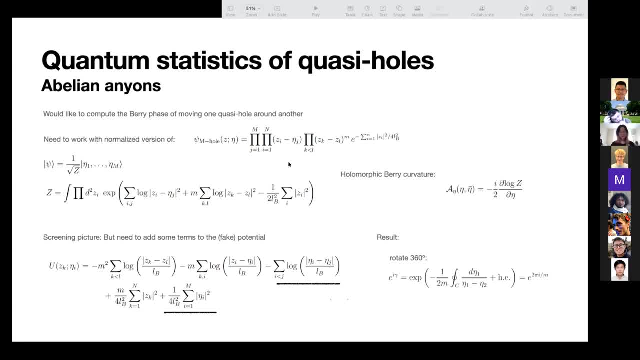 Yeah, so we can compute this exchange. We can compute the exchange angle by considering the barrier curvature of this wave function containing m holes, and you know, just move one hole around another one to get to the statistic angle. But a caveat is that in order to compute the barrier curvature, we need to work with a normalized 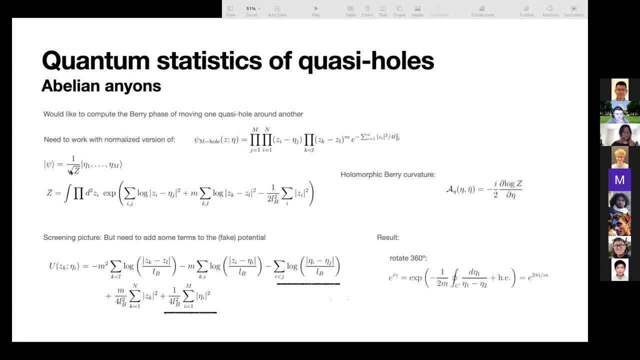 normalize the version of this guy, which is this one where c is just this partition function. we get in the plasma analogy, Yeah and right. again we want to use again, we want to see what a plasma analogy can teach us. So this whole system looks like we have some kind of defects and also a uniform background charge. 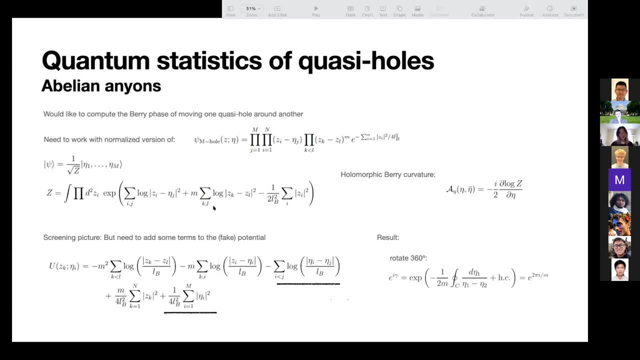 and the Coulomb interaction between particles. There's a Coulomb interaction between particles, Coulomb interaction between particle and defects and a Coulomb interaction between particle and charged background, But that's not the whole Coulomb interaction. if we, if we're considering a system with with those charged defects, We are missing two terms. 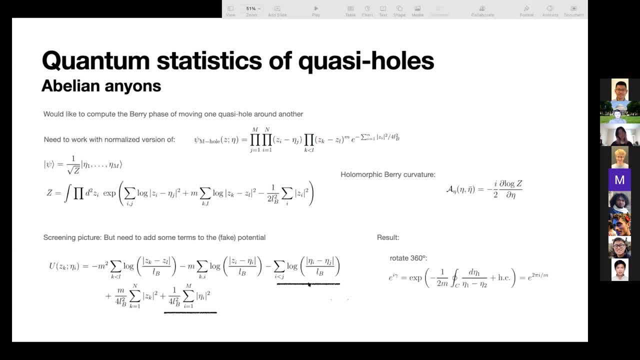 One term is the Coulomb interaction between the defects themselves. the other one is the Coulomb interaction between defects and the charged background. So if we add those two terms, it looks like. it looks like. So this corrected potential actually describes the whole Coulomb interaction energy containing these defects. 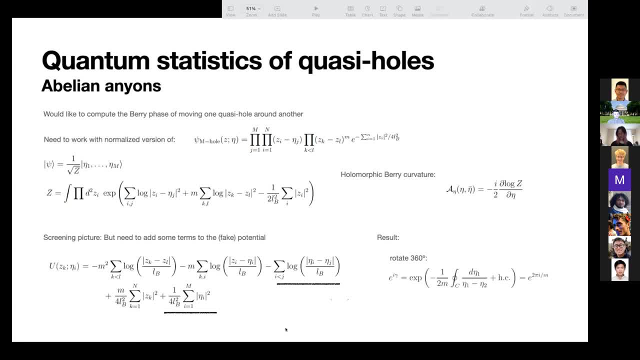 So yeah. so, as I said before, the whole purpose of the plasma is that they want to be neutral. So, yes, so if the total stuff is neutral, then it doesn't matter where I, it doesn't matter, It doesn't matter where I put those defects, they will be screened. 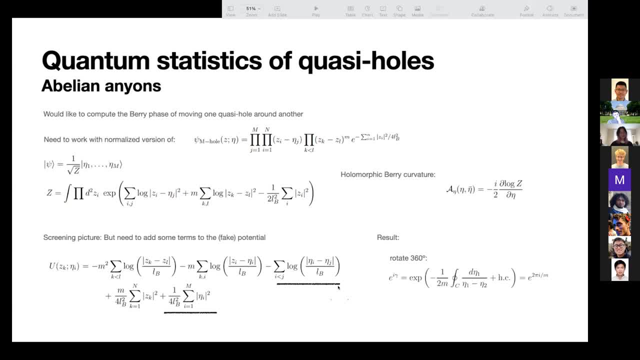 So that means actually, if we consider this corrected potential, if we replace this corrected potential, replace the original potential by the corrected one, the resulting fake partition function will be well they it. it doesn't depend on the position of eta. 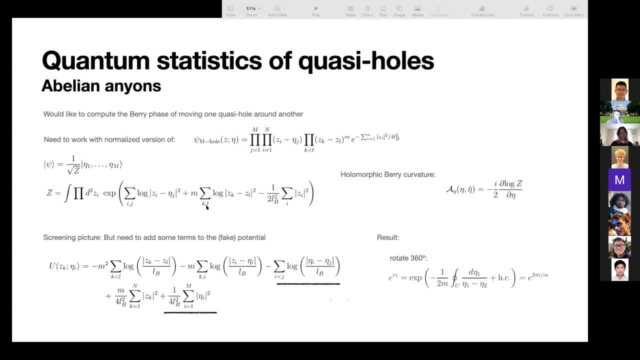 So that means the, the, the, the baric curvature of of this guy actually vanishes. So we only need to consider the effect of this, these two underlying term to the baric curvature. Yeah, this is much. this is much easier to deal with because they, because we don't need to integrate over those C's. 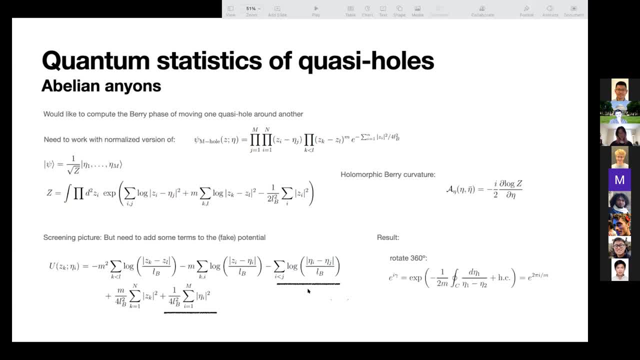 Yeah, this is much. this is much easier to deal with because they, because we don't need to integrate over those C's- And indeed we, if we compute the holomorphic baric curvature of this guy, we get some factor like this: 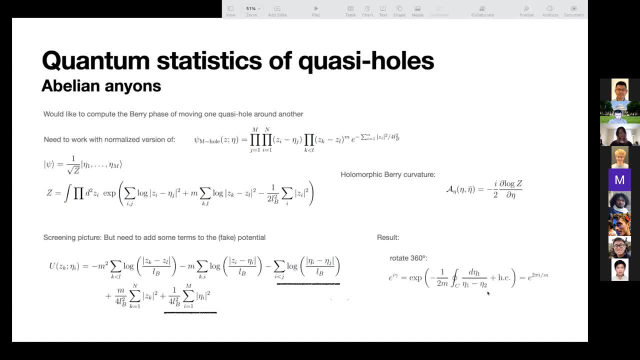 So if we rotate, say 1 RF², or投 waterfall around the other, rotate, say eta1 around eta2, we'll get a phase factor that's proportional to a two pi over M. Note that the statistic animals, meinz she- rotate to 180. 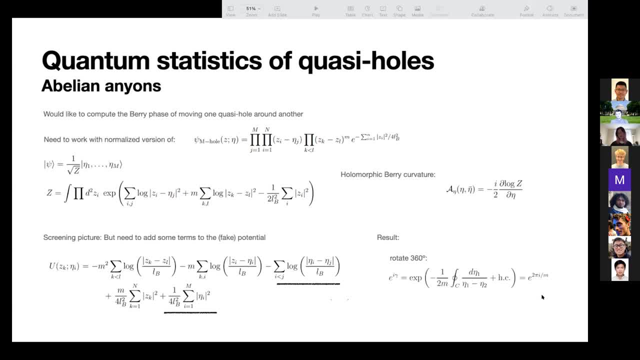 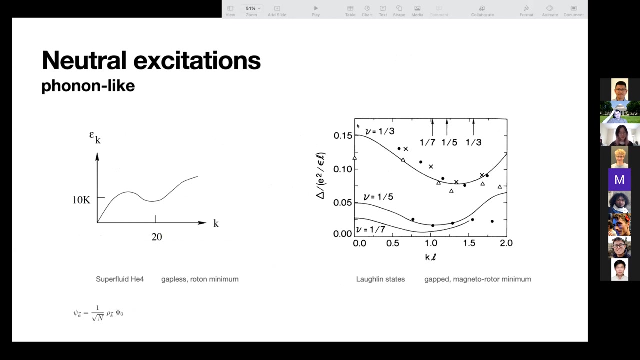 Not that the statistic angles is actually rotate to 180.. 80 degrees, not not to pack, So the statistic angle is one over m. So, yeah, Okay. So so so far we've been dealing with a charged excitation. I also want to mention and bypass we in those. 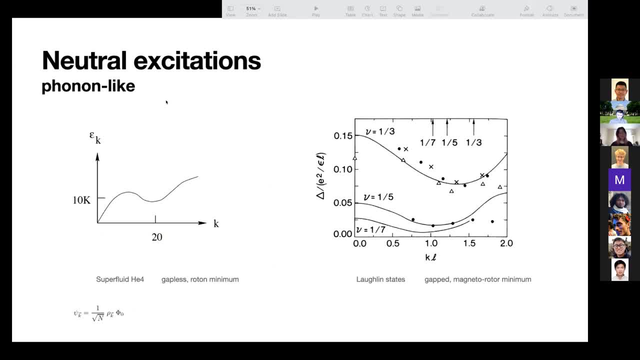 in those systems There's also a neutral excitations which are funnel like it comes from density fluctuations. It's similar to what happens in superfluid helium, for, But major difference between the superfluid and quantum Hall fluid is that the the phone on distribution is the full is gapless and superfluid, but it's a gap. 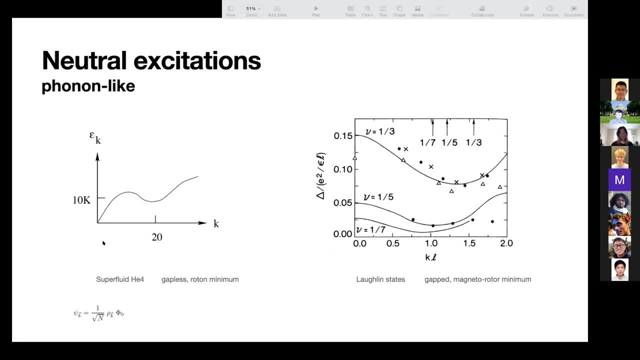 And a quantum Hall system, because then superfluid is a ghost on mode. but but this quantum off with actually it doesn't have any ghost on mode, etc. And analogously does also a Rotom minimum in this, In the quantum Hall fluid, Which people call a magneto Rotom minimum. 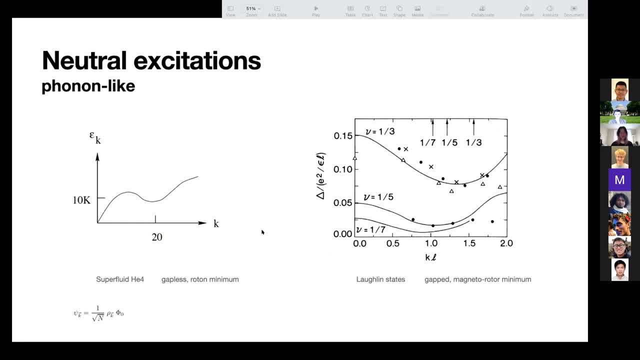 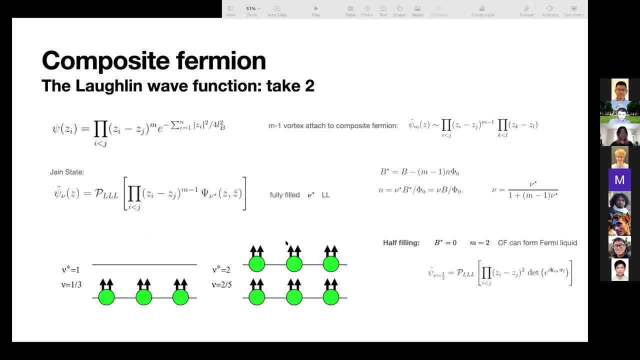 Yeah, if, yeah, if I have, if I have time, I can talk about how to get this more. But yeah, let me just skip the neutral citations. Okay, so far we talked about a lovely way function and the plasma analogy to it, but actually we can view a lovely way function from from another point of view, which is the point of view of composite for me. 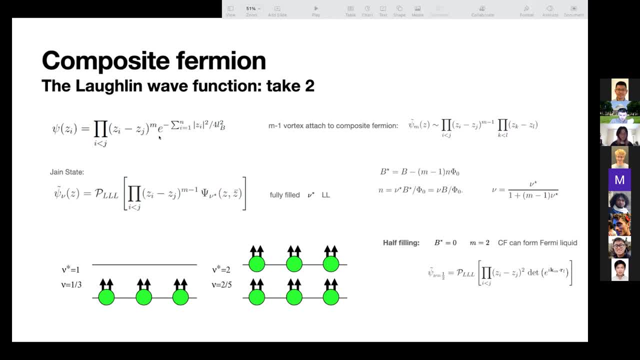 How does this work So? So the lovely way function is this guy And if we decompose this, this factor, to, to M plus one, power of M plus one and power, and what this? this second, The second guy looks like And times this exponential coefficient. It just looks like a fully filled lowest on the level wave function. 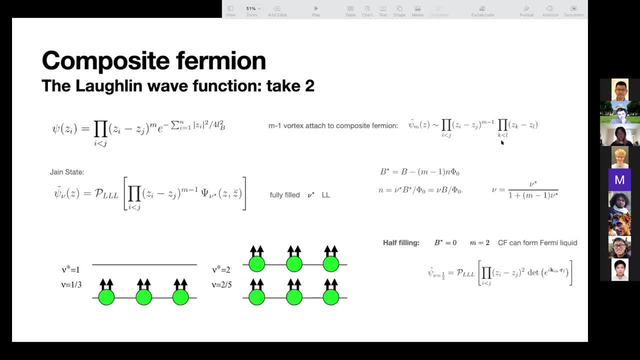 So, And- but I mean intuitively, is this lovely way function? just look, looks like we attach to this. see another vortex Of power, M minus one. So this motivates Jane to write some states like this, like this guy where this Poseidon new star is. 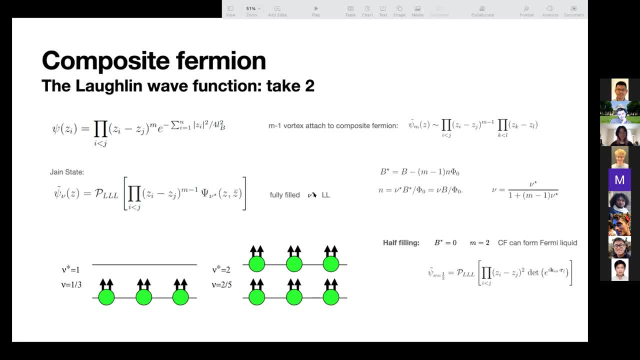 Where function of a fully filled new starts locked on level In in the. in the case of lovely way, function is new stars, one And attached to it Some M minus one flux And And after that we need to project the whole thing back to the lowest level. 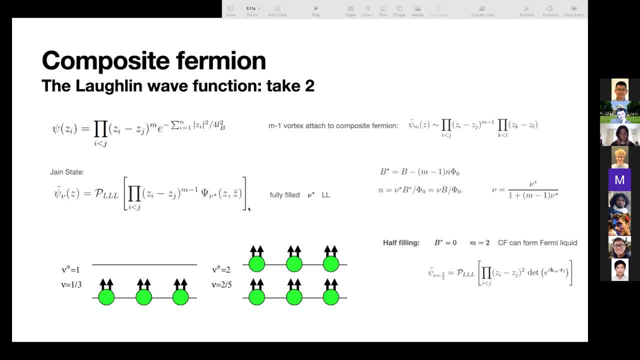 Because in this fully filled, if noon star is not one, there will be some anti-holomorphic part that's not allowed for a wave function in lowest lambda level. um, okay, uh. so let's see what this uh, what this composite for, uh, by us, by the way, we call this, we call the uh from, we call the fermion in this, new in this. 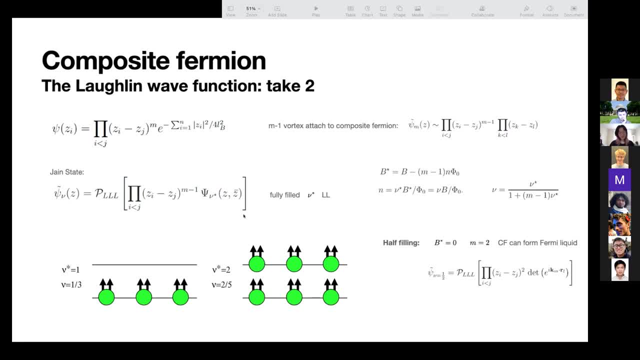 new star lambda level composite formula. so, uh, let's see what this composite formula picture can teach us. so, yeah, so uh this. so, first of all, this, uh, new star, the fermion, the formula inside this, uh this, uh low, this lambda level wave, function it, it should feel a different. 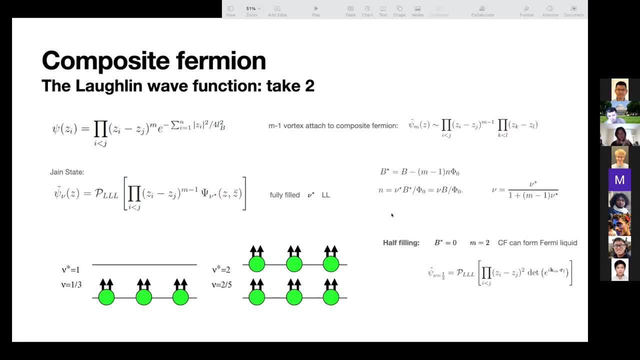 magnet magnetic field because we attach vortex to to it to get to get back the original one. so yeah, so actually the uh magnetic field field, magnetic field felt by the composite fermion as the original magnetic field, minus the m, plus one, which is the uh stress of the vortex times, the uh like the density. 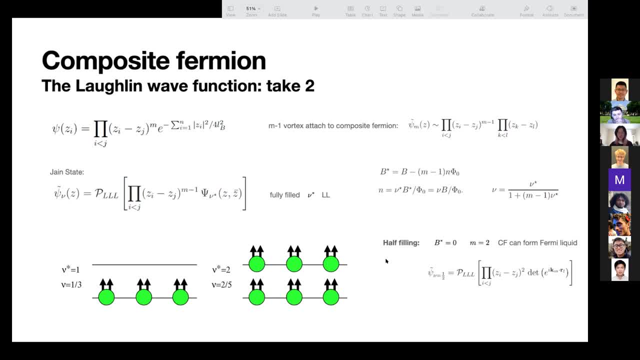 density of the those guys. so and also the uh. for each uh composite fermion we attach m minus one voltage, so the charge dance. so the particle density of the composite fermion and the particle density of the original guy should be the same. that allows us to determine a new uh feeling. 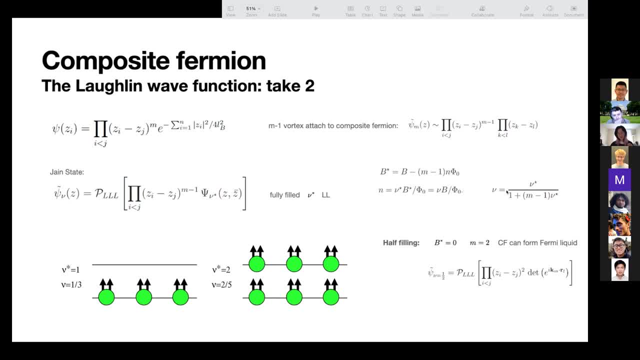 fraction, which is this new star and related to the original one, so yeah, so the relationship between a new star and new looks like this guy. we can pick any new as well- as it's an integer, so this gives uh and an m is also integer, so this. 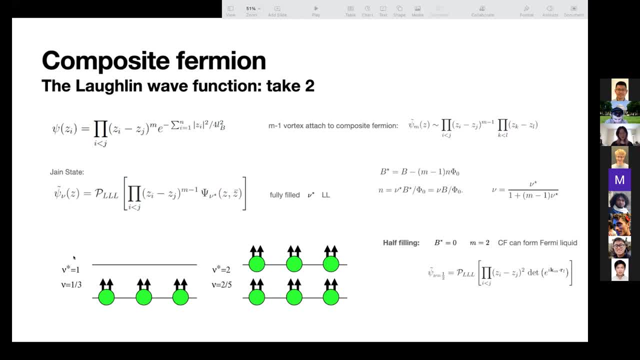 gives gives a whole sequence of wave functions which are called uh, which is called jane c jane sequence. so we can look at some examples. for example, if, if we, if we attach uh two, say m equals three, that means we attach two vortex to and to a fully. 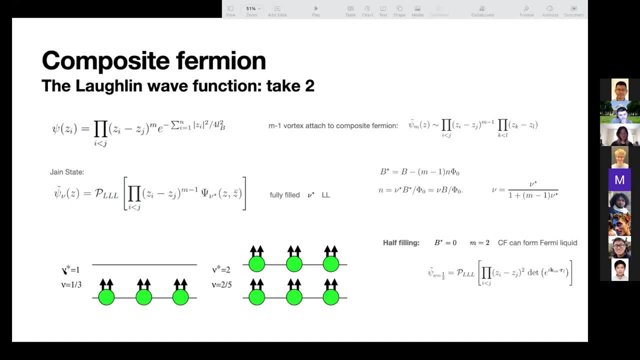 filled uh zeros, for if you're first level, new star equals one, a zero level, actually. so. so we'll get a new equals uh one over three, which is the uh, which is which indeed gives the uh right feeling factor because, remember, for the Laughlin state, 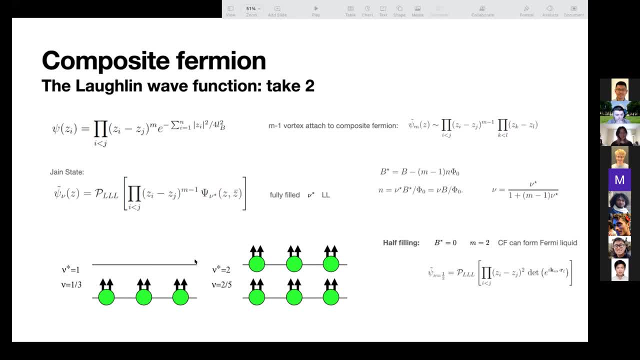 if we have the filling pressure one over M, and this can also be reproduced by this, by considering composite from you. Yeah, actually, there's a very interesting example to it is if we consider M equals two and this B star equals zero. 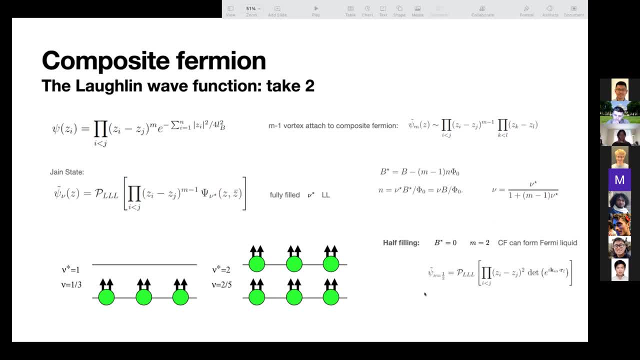 that will give a half filled Landau level. But notice that this wave function is actually not correct for that half filled Landau level because the magnetic field- of the magnetic field that's filled by the composite formula, is actually zero, So the composite formula can form liquid. 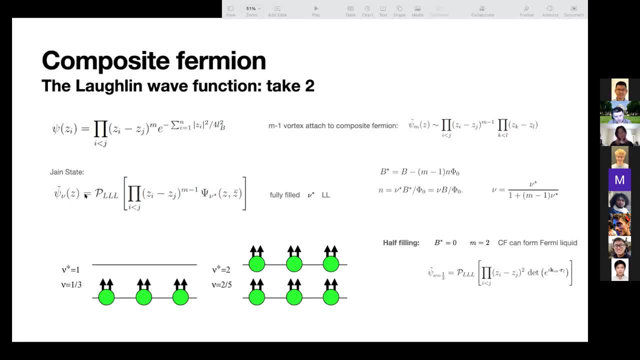 so instead of this chain state we can write a new equals half state, like this guy, where this determinant is just a wave function of Fermi liquid. Okay, that's good. Another question: So I sorry, I just can you remind me why the lowest Landau level has no Z bars? 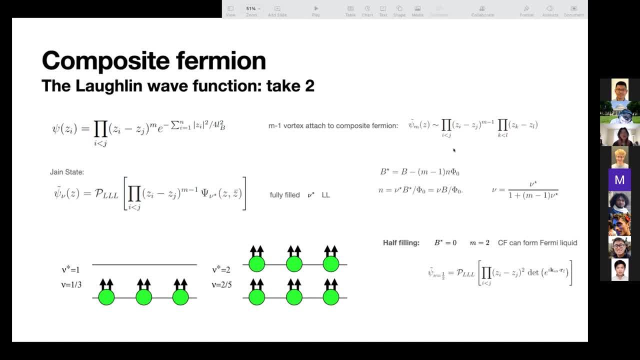 I forgot. Oh it just, it just comes from the symmetric gauge. If you choose a symmetric gauge, then the lowest Landau level wave function will always be a holomorphic function. times some coefficient, Oh, here I just. I mean, here I didn't include. 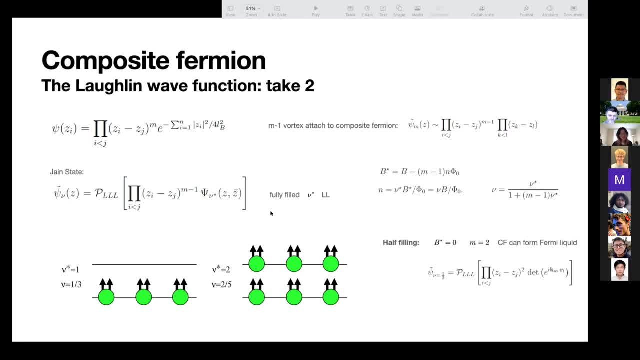 any that, the exponential factors. But okay, so that follows from the Hamiltonian or something That that boils down to versus. of all, the energy scale problem is the coulomb energy much less than the ladder level splitting, So Uh huh. 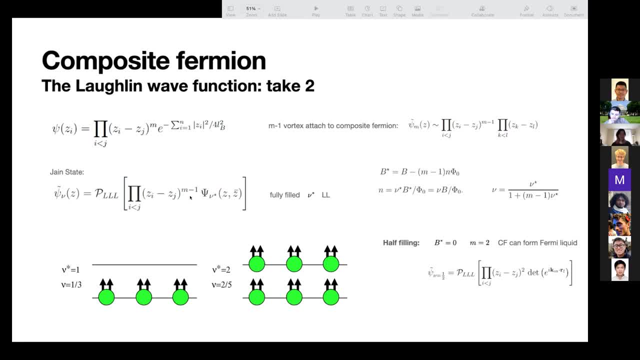 So we can- just consider the projected Helmer space spanned by the wave function of the lowest Landau level of the non-interacting Hamiltonian. Yeah, OK, And so the claim is that if I were to write a z bar and psi. 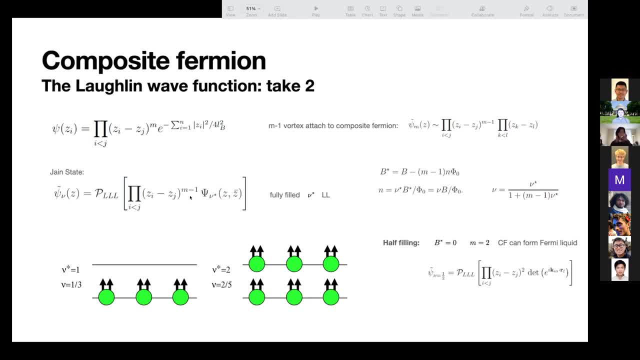 or something. what would that be doing? No, If you do a projection to the lowest Landau level, it will give you something like partial z. OK. so the rule for implementing this P-L-L-L thing: if I have some z bars in psi, I try. 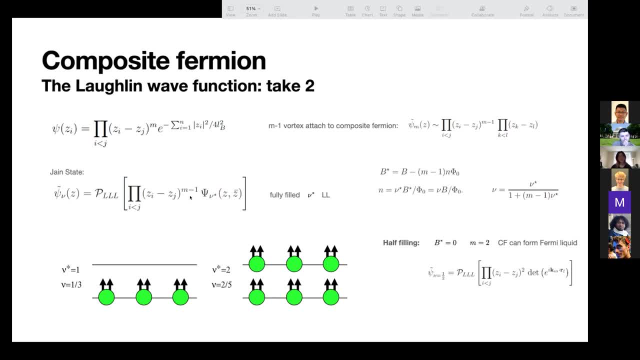 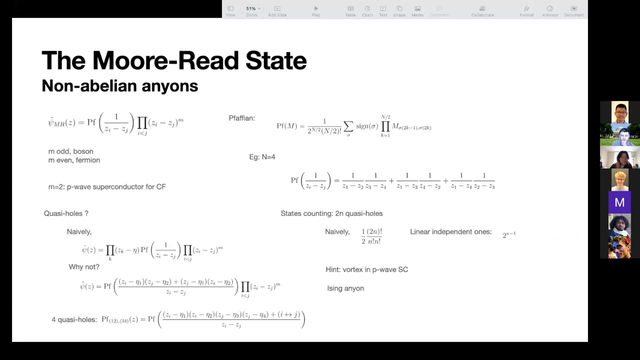 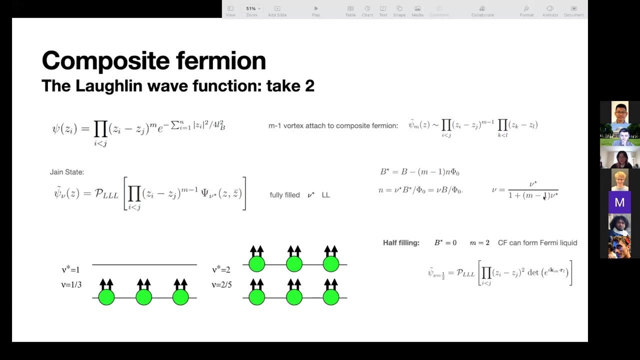 to replace them with derivatives, as you did earlier when you were describing the quasi-particle wave function. Yeah, yeah, yeah, yeah, with derivatives on this factor. OK, I see. Yeah, any other questions? OK, yeah, so this Jane sequence is very nice. 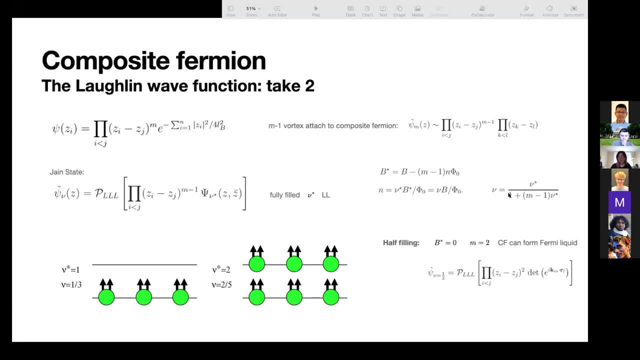 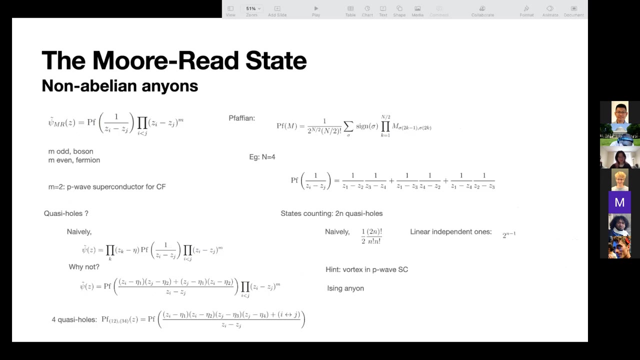 but it only gives rise to a certain kind of the filling fraction, which is with odd denominator. OK, Yeah, OK, OK. So in the spirit of guessing ground state wave function, we can try to do more, more than a Laughlin wave function. 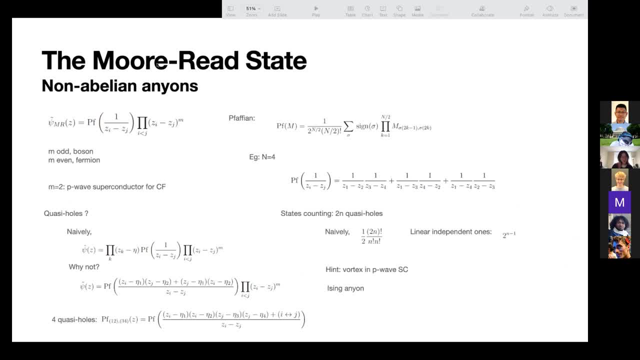 So, yeah, that is so more. I really propose this kind of states. So this: I ignored the OK Exponential factor, So this more read state is very has a very peculiar form, with a far fear in front of it, So sometimes so it's also called Fafian state. 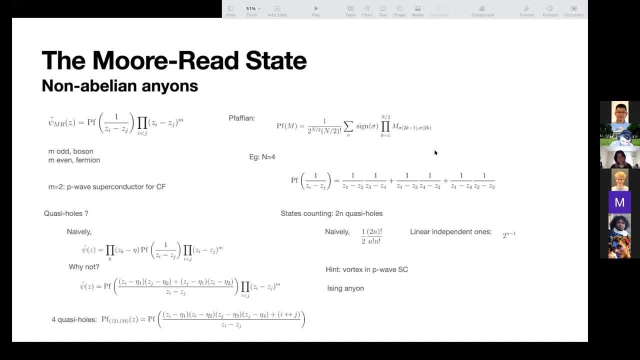 So the Fafian is something like a square root of determinant, which is defined by this expression, Right, So yeah, So let's first look at a single example. if we have n equals four, So the far field of this guy with four particles can be written as something here. 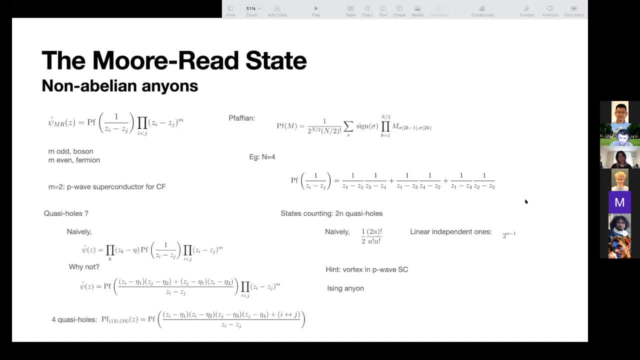 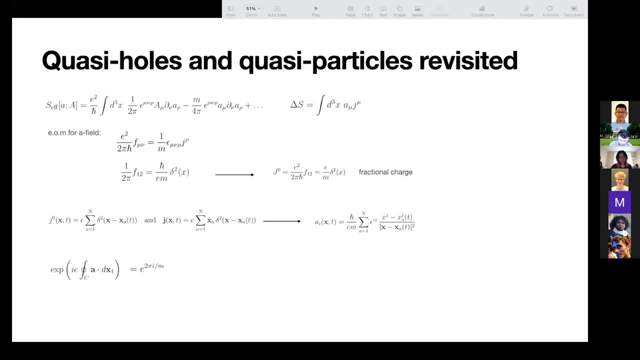 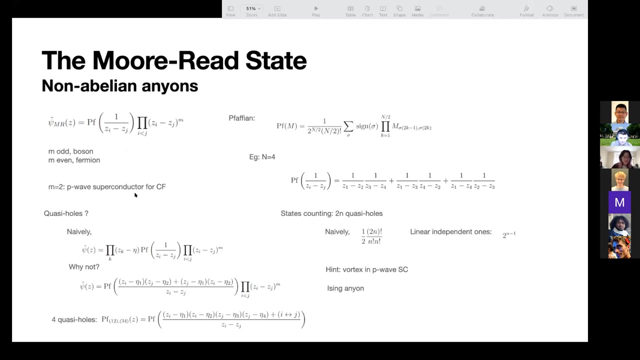 So basically we just partition four particles in terms of two particles and two particles and exchange indices With some sign of the permutation. Sorry, Yeah. So this far field coefficient times, this guy, Yeah, it actually doesn't have, actually doesn't have any divergence when ci approaches zj. 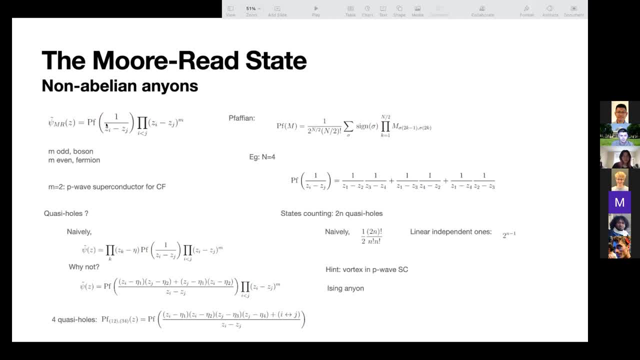 So this is, This is very good, And also because this far field is naturally is anti symmetric, So so there's more real state is for bosonic system where m is odd and for fermionic system where m is even. So. that's a difference between this guy and the Laughlin wave function. 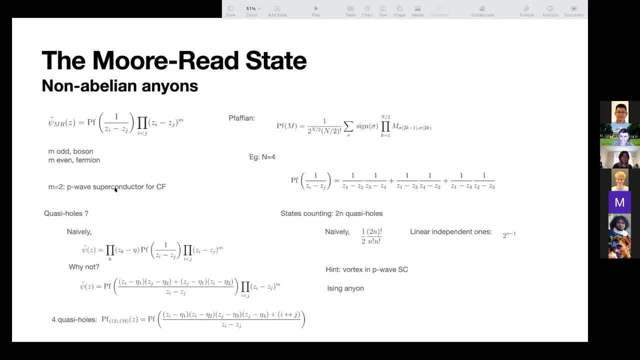 So interestingly, actually for m equals two. this describes a P wave superconductor for the composite fermionic system. So we can also consider the quasi-hose for this wave function. So, naively, we will just include this pre-factor in front of the far field for one quasi-hose. 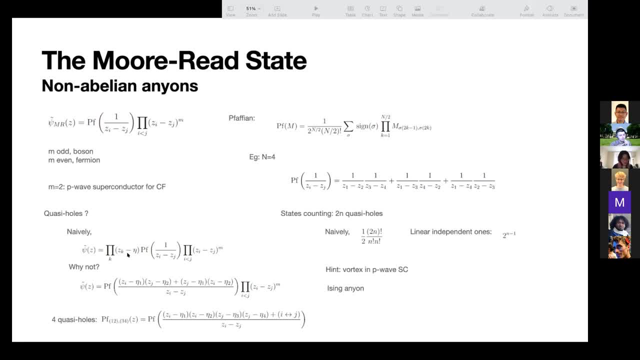 But But what? why? why not we do this? we we can, We can write some something we can mess, We can mess up with this far field coefficient and and put the, put the, put the, put this coefficient inside the far field stuff. 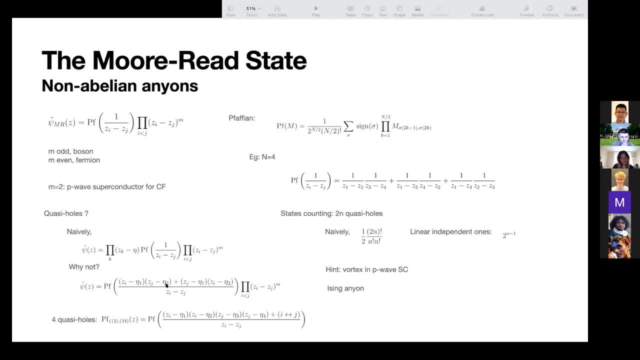 And you can see that when eta one approaching eta two, this guy, this guy is proportional to this guy. Yeah, Yeah. So that means That means we actually have. We did this. this hot, this putative half hole, actually putative quasi-hose, actually splits into two, two quasi-hose. 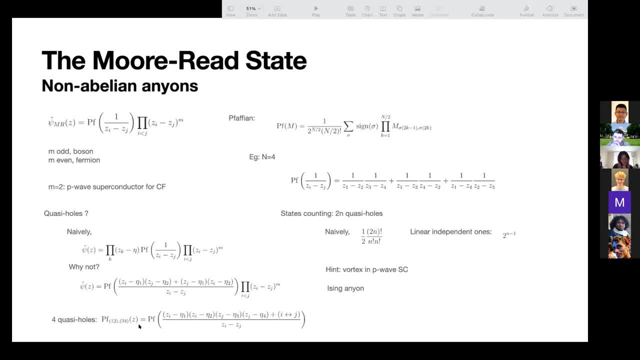 Yeah, so that that's very interesting And we can include more quasi-hose in terms Of the coefficients on the numerator of this far field. And So now we want to come count how many states there are, if we have to, and call that host. 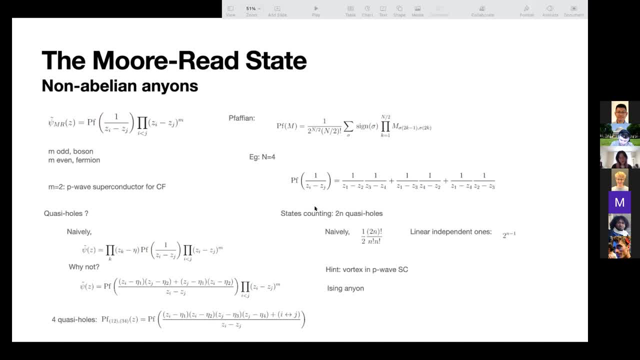 So naively we divide, We divide to and call that host into two piles. So naively we had, we will have this Much Of This many states, But Actually those Far fear are not Linear independent. So the linear independent ones are only. 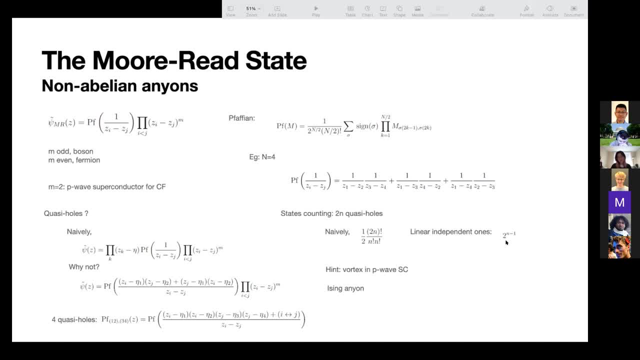 Two to the minus one, Much smaller compared to the naive counting Yeah. So Why this happens? So, As I mentioned by, As I mentioned before, actually this M equals two is P wave superconductor for composite fermion. 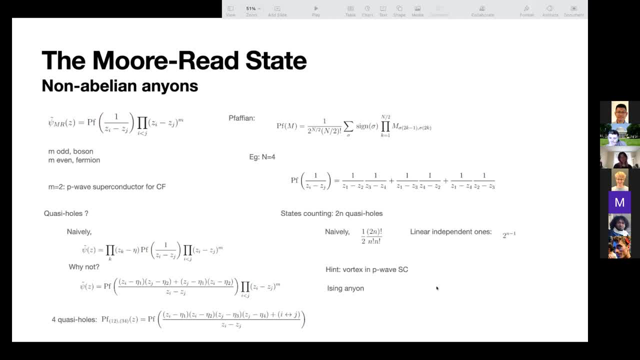 So This quarter, these quarter holes are actually vortex in a P wave superconductor. So If we come, if we, If we compute the, The, The bounce, The bounce state Of the vortex In pure superconductor. 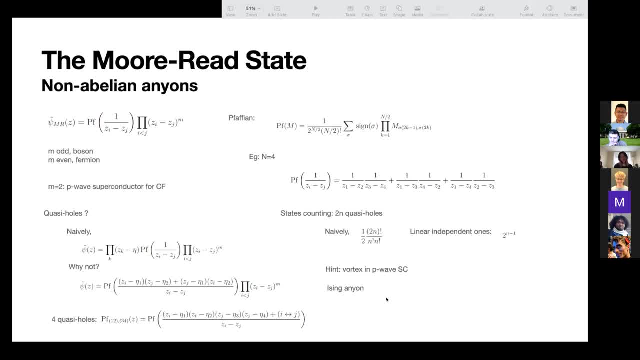 We will find that it's actually My Rana Fermion, So that If we have Some my Rana Fermions, So I mean we'll need two of them to form Complex fermions and Such that we can have. 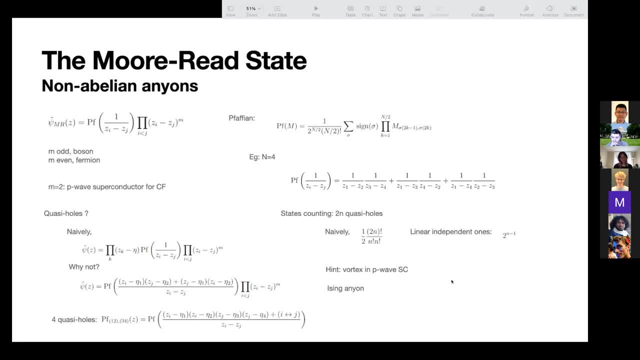 Two States, Such that we can have This complex when we are occupied or not occupied. that spans a two dimensional helper space. So that's why. That's why we get This Bizarre, Bizarre number of Linear independent states. 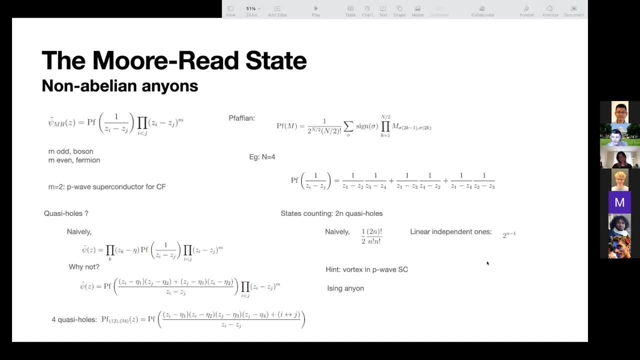 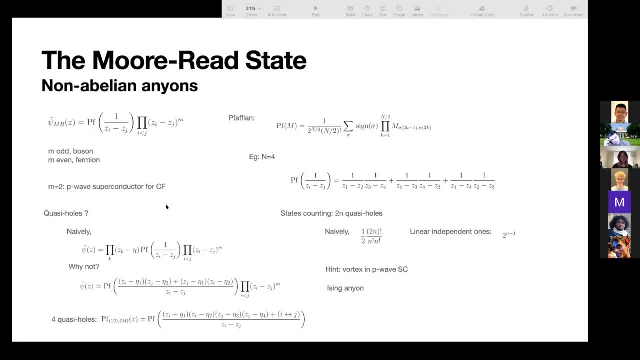 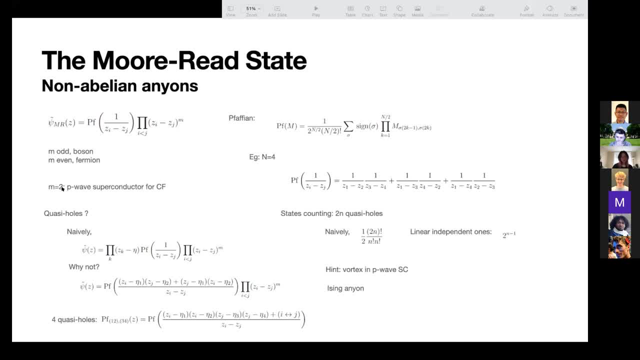 Yeah, Yeah, And These, These, So, but we'll find that I probably will not have time to talk about it. It's actually called Ising annuals, So yeah, so so far this- those wave functional approaches- looks good. 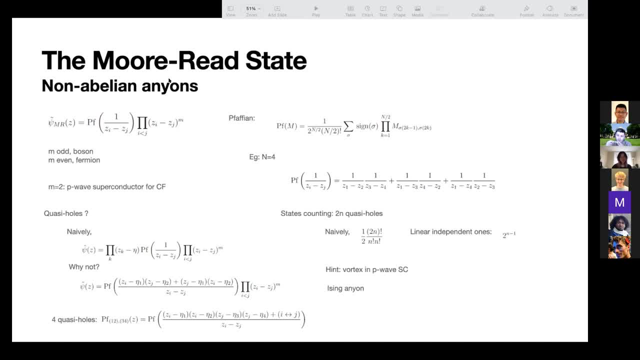 but when we, but when we are dealing with states like more restates, this wave function looks very complicated and it's not, it's not at all obvious how we can obtain the statistics of the quasi-hose Right if we want to, if we want to. 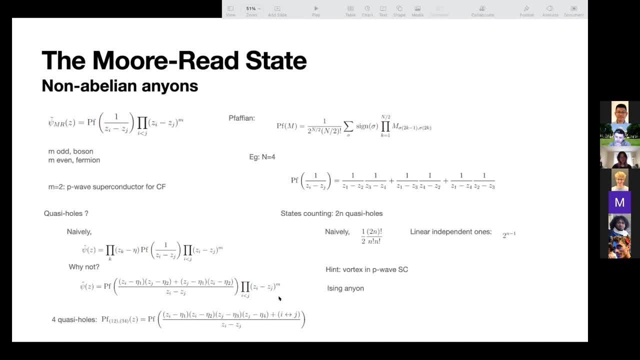 if we want to compute, say, just the space, just the space of the, just the Hilbert space of the quasi-hose, it will take a lot effort to try to analyze those Fafia coefficient. So so an alternative way of dealing. 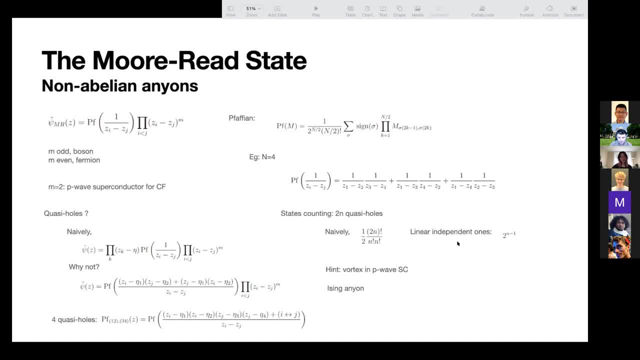 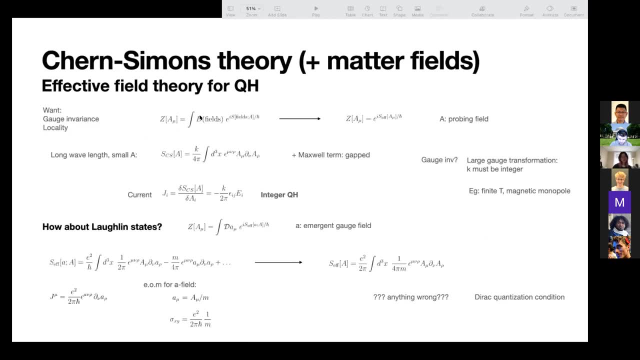 with fractional quantum core is we sort of take a coarse-grained approach and think and think of what kind of effective field theory? what was the effective field theory for a quantum hole? So by effective field theory I just mean, since the quantum hole, the quantum host, days are gap to. 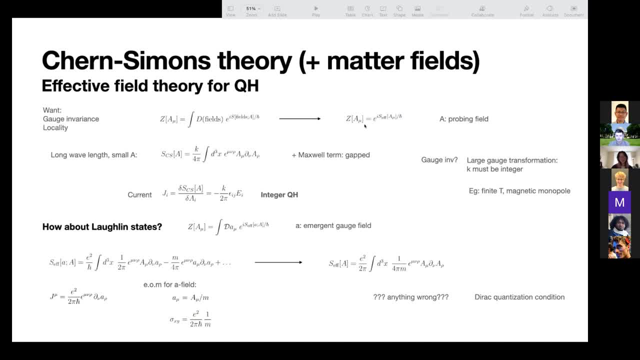 we can just integrate out those smattering fields and get some effective action with a background gauge field where the gauge field is a probing field. It's not the original. the original, you know the you know the original magnetic field that caused the quantum Hall state is not included in this. 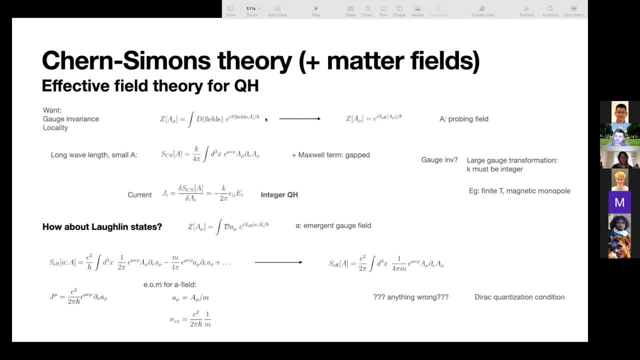 big A. So from a general consideration of reasonable field theory, we required the theory to be gauge invariant And so we also wanted to be local, And we're also dealing with probing fields. so we want an effective theory at long wavelengths and relatively small gauge. 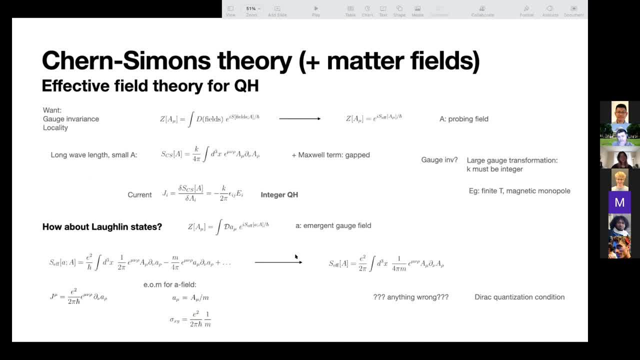 fields. So there are not many terms we can write down, and we can write down them order by order because we're considering this limit. So the leading order term is called the Transimons term, which looks like this guy, And the next order is the Maxwell term. 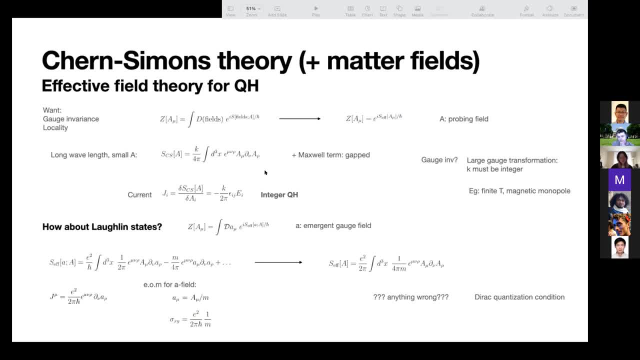 So Okay, Yeah, so the Transimons term plus Maxwell term actually gives a gaped photon spectrum. So it's good because we want to consider gaped theories. Also, if we compute the current of this probing field, it actually has a Hall coefficient, which is also nice. But one puzzle: 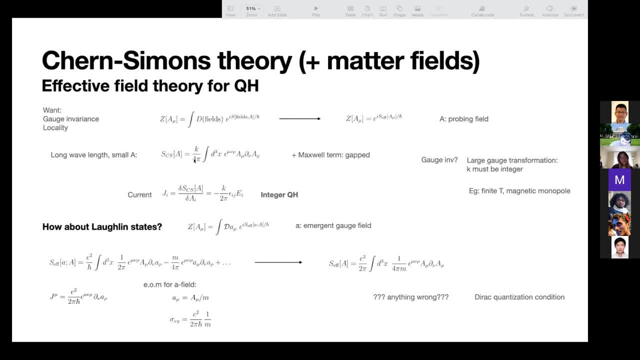 is that this Transimons theory seems to be a little bit different. The Transimons theory seems to be gauge invariants, So I mean there seems to be no constraint of this Hall coefficient. So how can we relate it to integer quantum Hall? So actually if 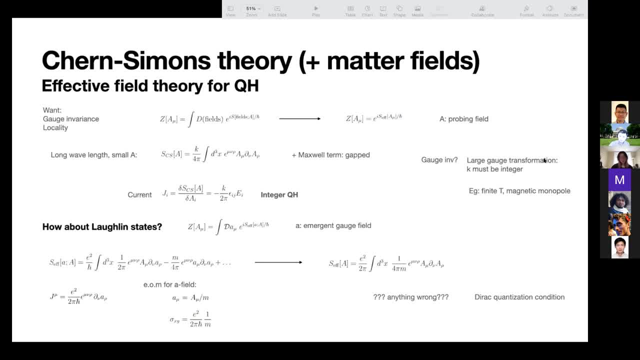 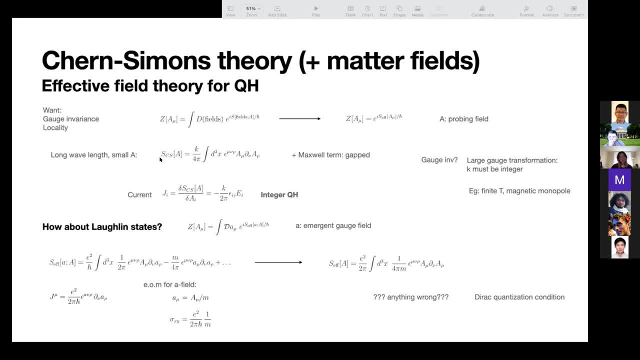 Right. So the large gauge transformation. one thing to consider is that we can put this system, We can turn on the finite temperature, meaning we can do a weak rotation to Okay. So to consider a finite temperature configuration and make this also make the space compact. 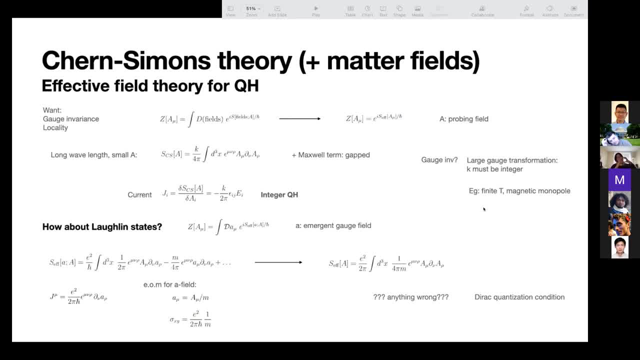 consider a a sphere and we insert a magnetic monopole to it. consider the whole path integral. Yeah, and we can for this. so the gauge invariant actually requires this partition function to be single valued. but this effects to action can have some face. 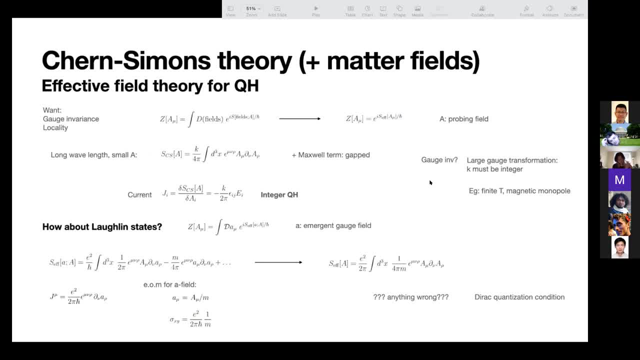 face factor. After considering that, taking that into account, we will find that k must be an integer. So, but as we talked before, we can have Laughlin states, which I mean the whole response doesn't need to be integer. 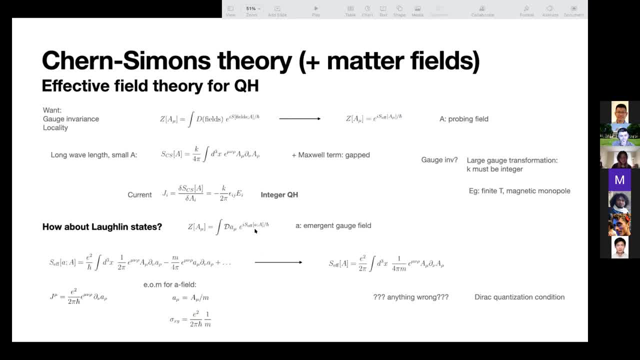 So what happened here? So let's put this aside and just consider another theory. with emergent gauge field coupled to the probing gauge field- And since now we know this trans-Simon's term is actually gauge invariant, we can introduce a trans-Simon's term. 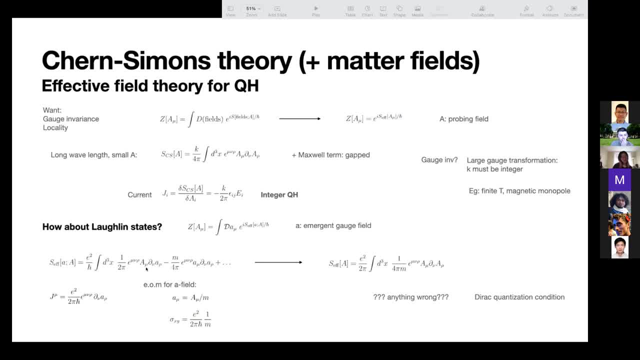 for the emergent gauge field and a couple and have a mutual trans-Simon's term between the probing field and the emergent field. So then the current of this probing field is given by this gap And automatically this, the current, is conserved. 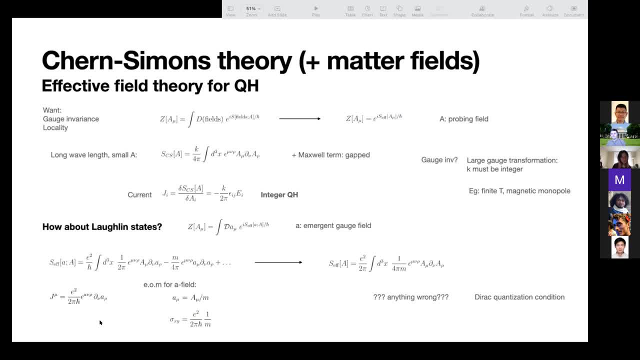 But if we consider the equation of motion for the little a field, we'll find that this little a field is actually one over m to the big a field, with some plus, some gauge stuff, And that's what gives. that will give us a whole conductance. 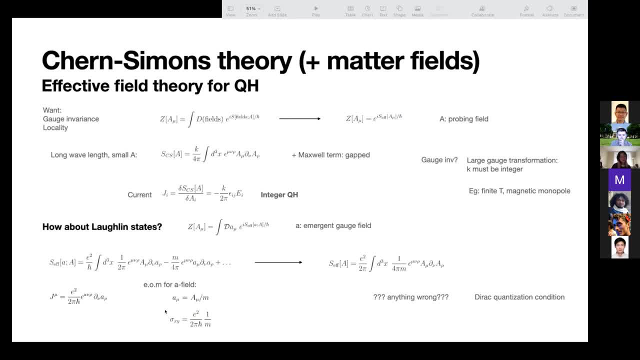 which is one over m, And if, furthermore, if we integrate out this little a field, we'll get a one over m coefficient in front of the trans-Simon's term. So that seems. that seems that conflicts with the observation we just had. 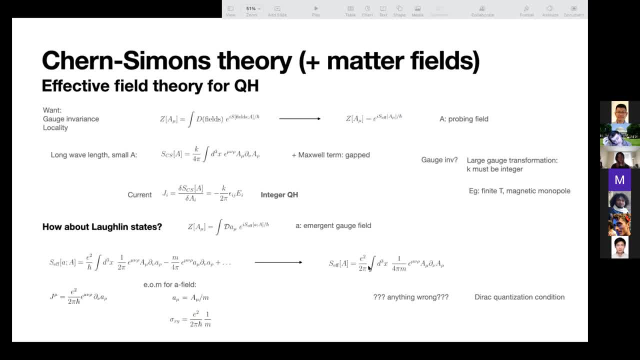 That means right we? I just told you this. the gauge invariance required this coefficient to be an integer. So so what's wrong? So actually there's. I mean, there's nothing wrong about this gap. The problem is with the Dirac quantization condition. 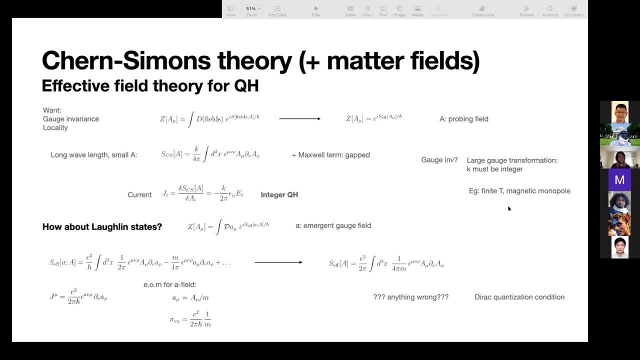 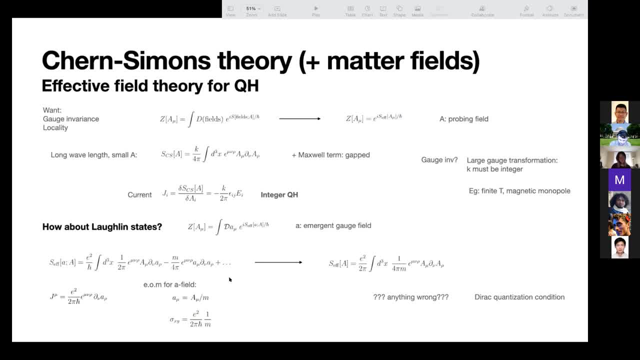 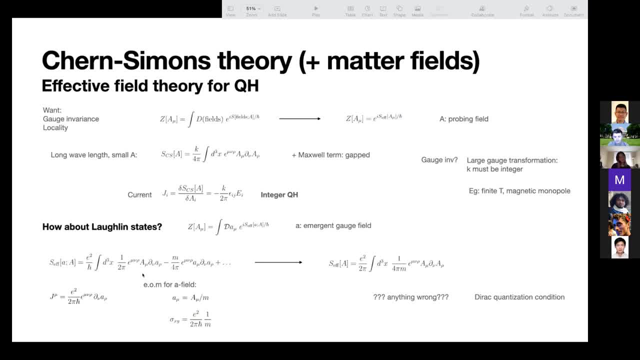 we have normal components in both parts, so you can часть by Dirac quantization Maybe, if it's, but here I actually require that Dirac quantization condition for the little a field, not for the big a field. That's why we get this one over m coefficient. 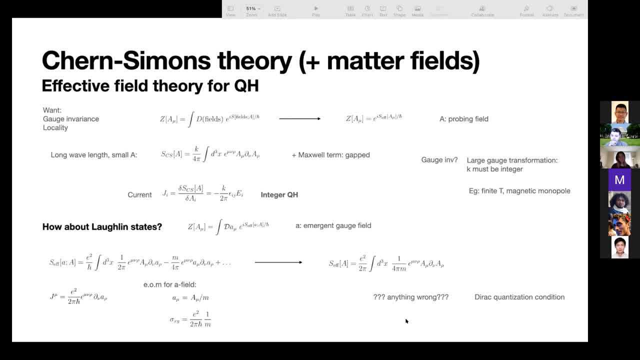 the coefficient is actually meaningless. We have to specify what we call charge one to. I mean to make those coefficients meaningful. Yeah, that's a caveat of dealing with Trensheimer's theories. Oh, okay, So from the Trensheimer's theory we can also 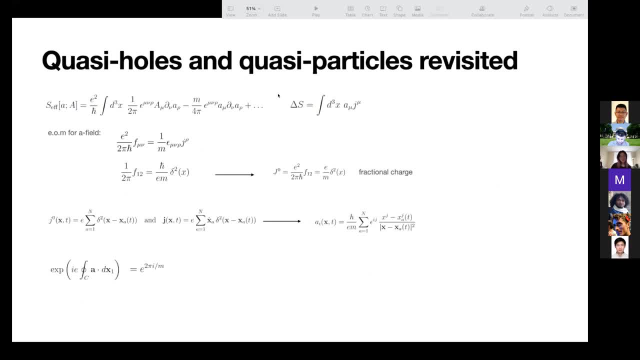 calculate the quasi-hose and quasi-particles. consider quasi-hose and quasi-particles and their statistics. Yeah, that's, I think that's if you, if you take Xiaogang's class, I think this is one of the homework problems. 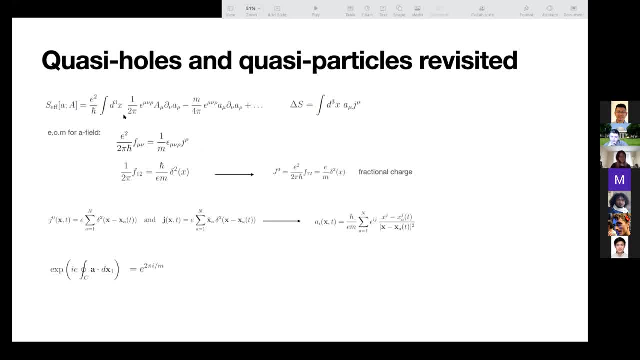 Yeah, basically starting from the effective action we had before and add some charge density to it. So, yeah, And if we consider the equation of motion for the little a field and so and turn off the probing field big A for a moment, we'll see that actually this charge of 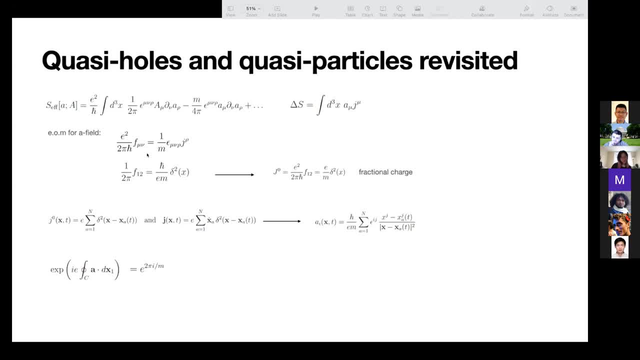 yeah, actually the charge, this, this electric charge, is attached with some magnetic flux of little a, So people often call this flux attachment. And if we plug the plug, the equation of plug, what we get from the equation of motion of little a field back into the definition of. 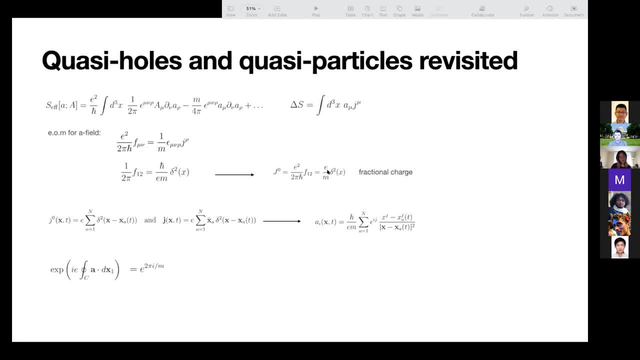 the current, we'll find we get a fractional charge. So yeah, So we can also consider the statistic angle of two, two quasi-particles, by writing, by solving the, by solving the equation or motion of little a field, and the compute and computing the AB phase of. 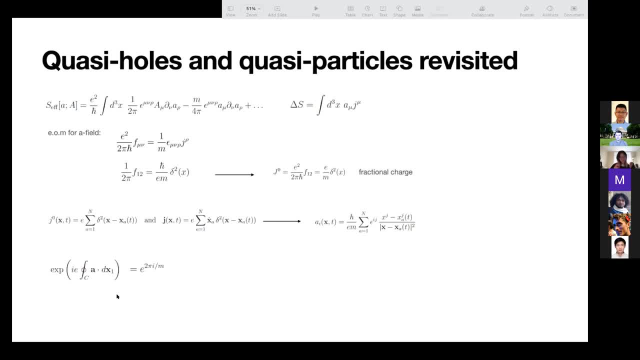 and by considering the AB phase of rotating one one for the whole around another, In the end you'll get the same result as we talked before. Okay, this emergent gauge field- considering these emergent gauge field- is looks like a very promising move. 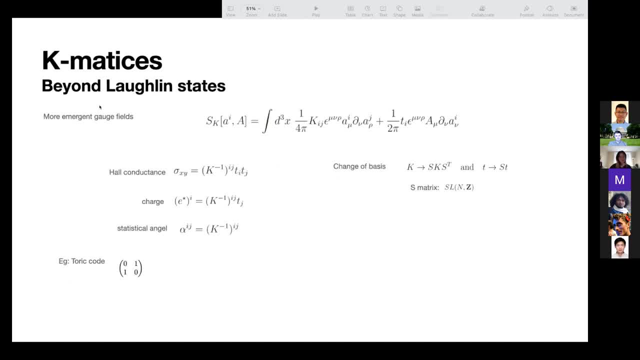 So why not have more of them? So we can have more emergent gauge fields and, in general, this effect, the effective action, will be like this guy. So we have a transcendence term between the emergent gauge fields and the mutual transcendence term. 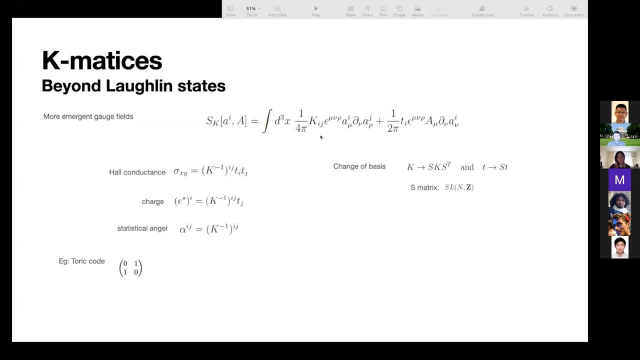 between the emergent gauge fields and the probing field And the coefficient. here is a matrix. People call this K matrix. So we can also consider the whole conductance, the charge, the statistic angle. Yeah, you can work out those by yourselves, I think. 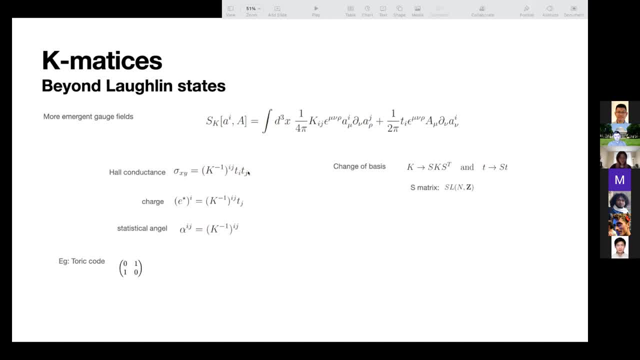 Yeah, and they all have this very beautiful formulas. Also, note that different K matrix and this T vector doesn't necessarily give, doesn't necessarily give us different states. So there's actually an equivalence relation. That's a yeah. So if we yeah, but note that we 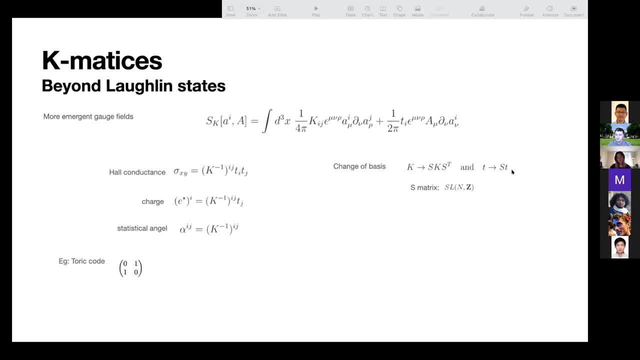 we also want to impose the Dirac quantization condition. So this equivalence relation is given by this S matrix with, which is an element of the SLNC, And the K matrix is the vanquished state. And the K matrix is the vanquished state. 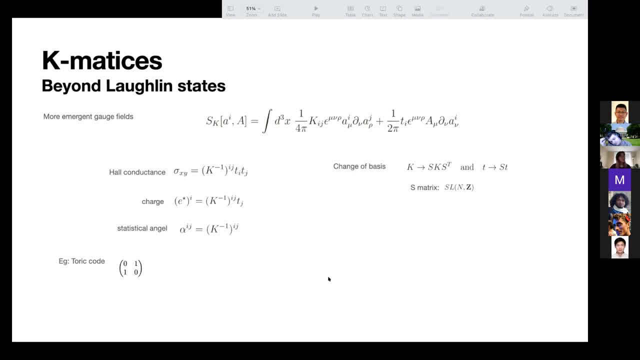 This is an element of the vanquished state And the K matrix is an element of the vanquished state. So if we can use that, the K matrix is very similar to what we saw in the previous work, The usual case. 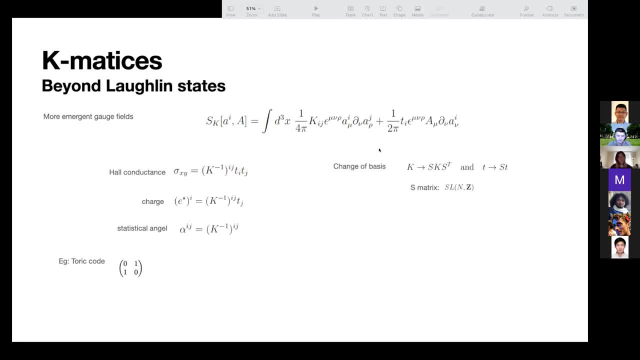 we have a very common K matrix with the same values. So if we just use, we can draw the other K matrix. Now topological orders, for example, such as toricode, Although I mean we can forget about this coupling. 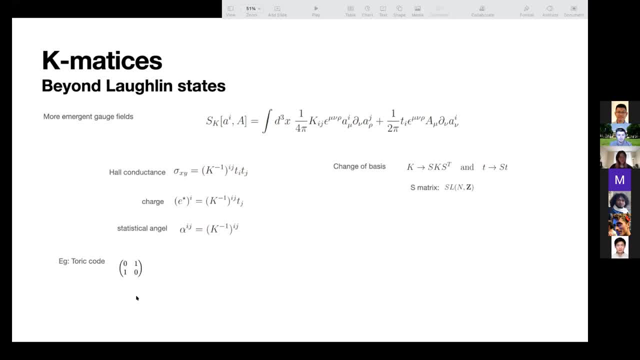 to the probing field for now. but for this K matrix, the K matrix for toricode is simply this guy. So we can check the statistic angle and find that E particle and M particle actually charged under this emergent gauge field, with a charge one zero and a charge zero one. 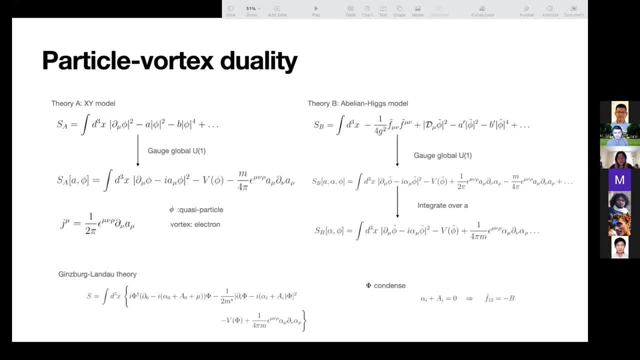 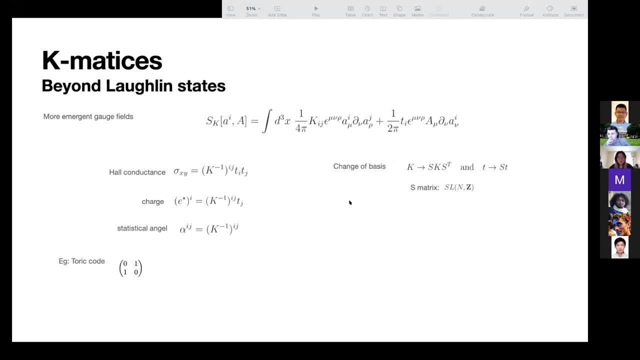 Okay, so we talk. so I tell you that this effective Hamiltonian can describe quantum pole states. but we can also put- we can also put the matter field back and make the. so this effective action is integrate over the matter field, So we can also put the matter field back. 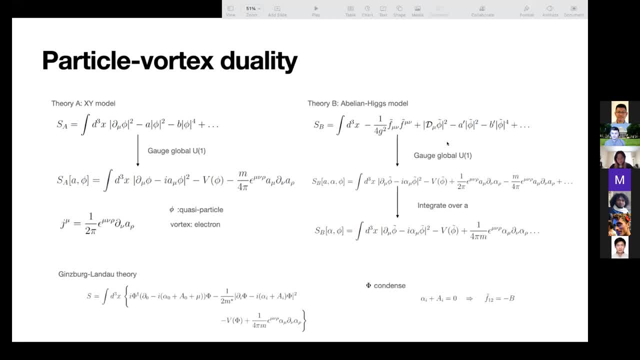 to see what happens. Yeah, and actually this, So, yeah, so I actually want to talk about the particle vortex duality. In the particle-vortex duality, on one side we have the S-Y model, on the other hand, on the other. 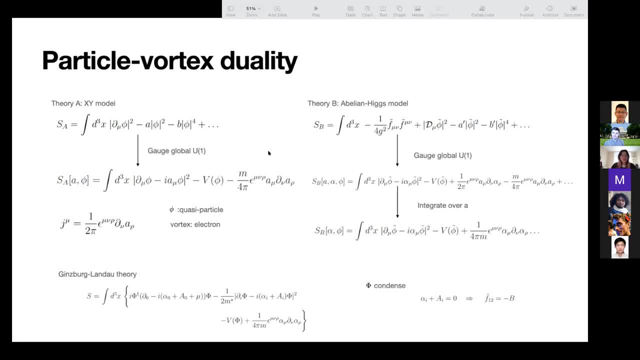 side we have the Abelian-Higgs model. So we have a global U-1 symmetry on both sides. and if we gauge that global U-1 symmetry with a dynamical gauge field, little a- and now we know that we can have transimers term as some gauging invariant terms- we can just 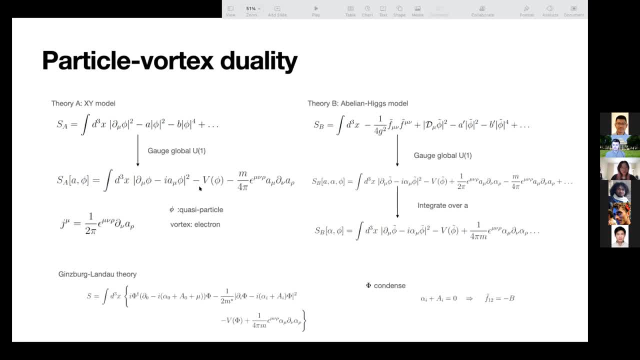 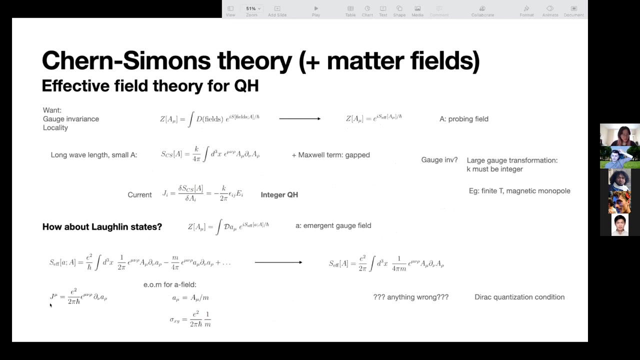 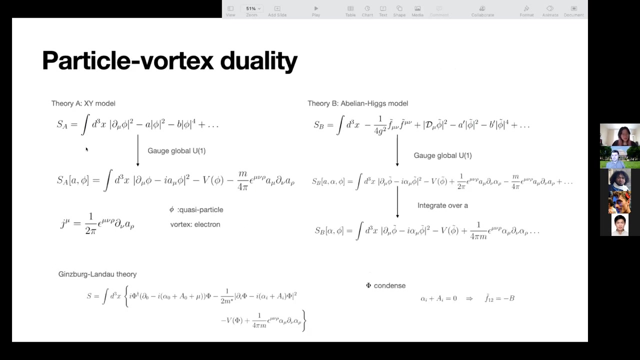 call the transimers term here and here. So notice that in this theory A, if we consider the current to the, so if we consider the current is actually given by this guy, it looks a little bit like it looks pretty much like the current we have here. Yeah, so that means in this description. 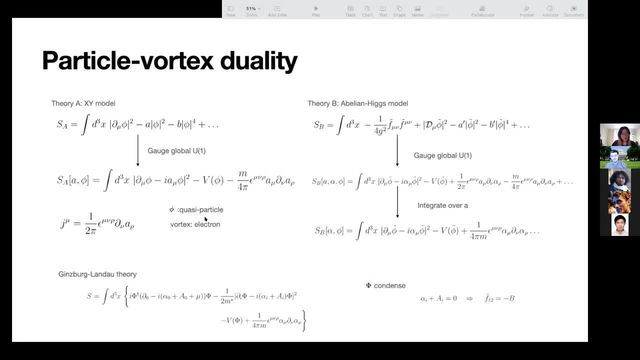 of this S-Y model. if we couple it to, we can also couple it to a probing field which I didn't write down, So yeah. so then this, this vortex is actually an electron and thus the phi quantize actually gives the quasi-particle. 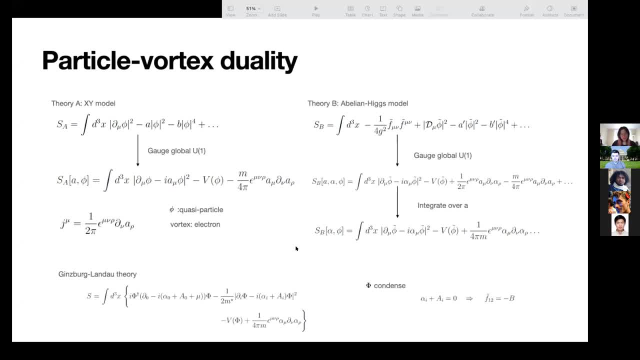 But we can also see that in the dual description, these, these two guys get reversed. So, Dan, let's see, I think we're a little over time, Sorry, No, that's okay, But yeah, so just like, maybe in five minutes, I don't know. 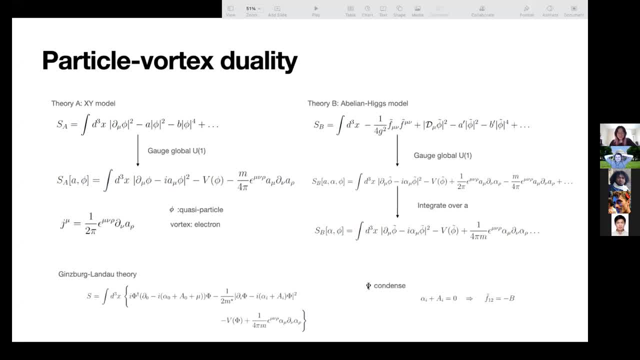 Oh yeah, yeah, sure, sure, sure, So, yeah. so we have considered the, the, the phase diagram of both sides, and and the work out, you know. so if say yeah and and match, match the phase diagram of both of the two sides. 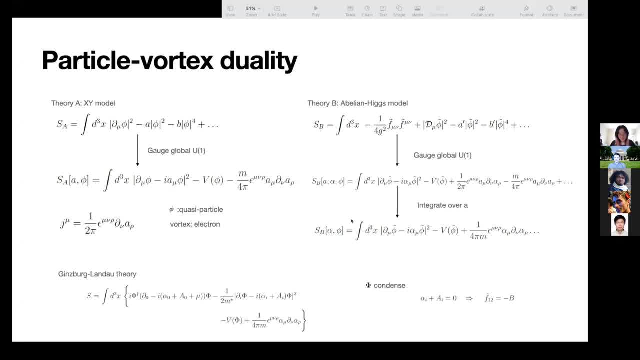 Also, I mean in this, in this language of particle, vortex duality. this phi field is actually has anti-particle And people also, and people in order, if you, if, if you want to get a Landau. 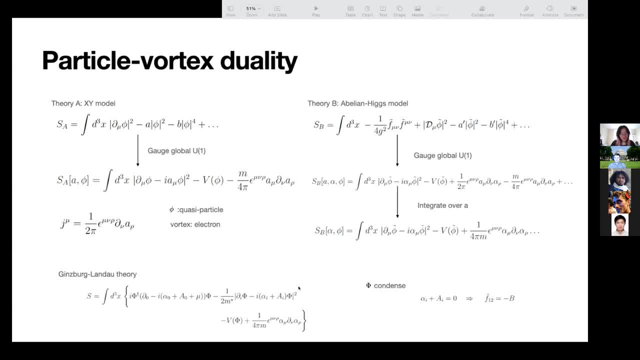 Gainsborough-Landau theory, plus the translammasome, you need to consider actions like this guy. Yeah, Yeah, Yeah, Yeah, So we're we're no notice that we replaced that here. this phi is relativistic and here: 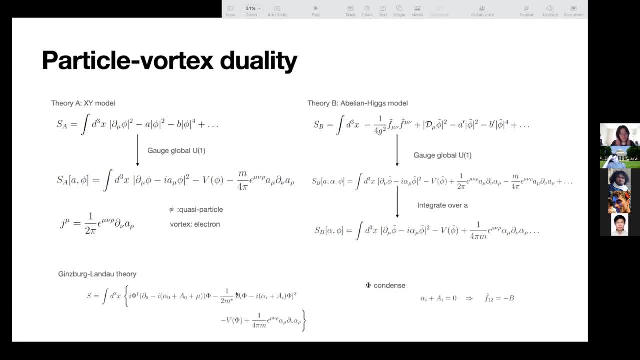 this little phi is actually non-relativistic and we put a chemical potential to it. Yeah. So I mean, at near critical points of this superfluid insulator transition, these, these two theories should be, should have same Sure. 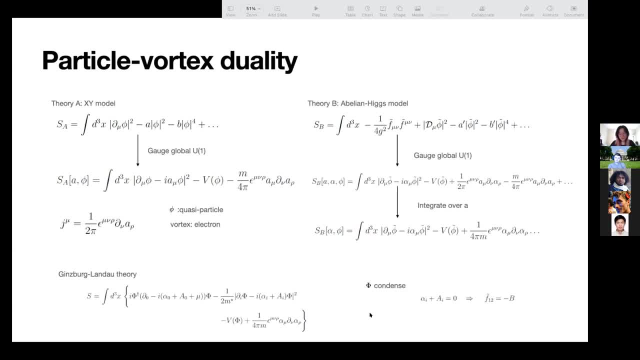 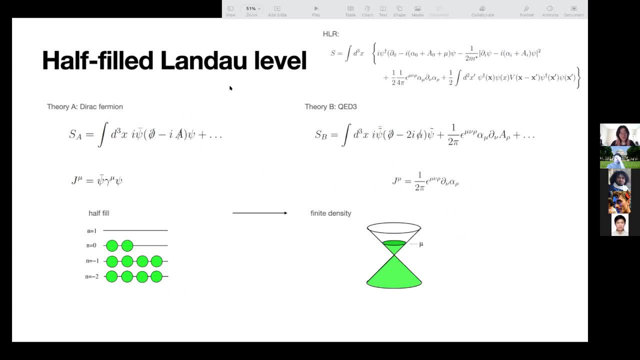 should be the same. yeah, And we can also consider half field landau level and a couple of yeah and do the duality, But yeah, but it will be a very long story for this half field landau level, so I'll stop here. 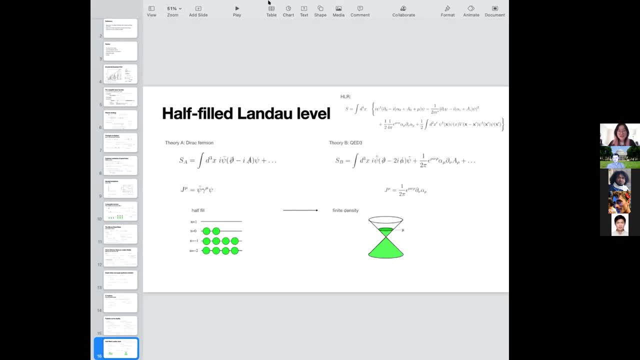 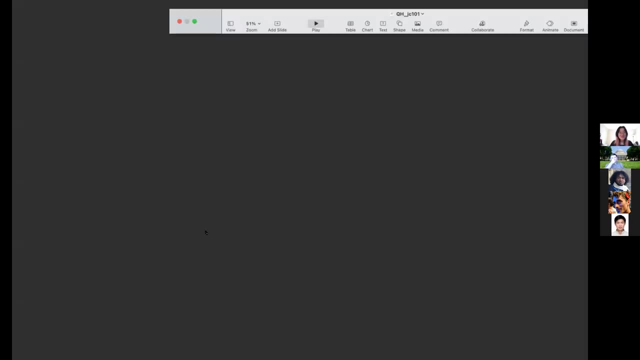 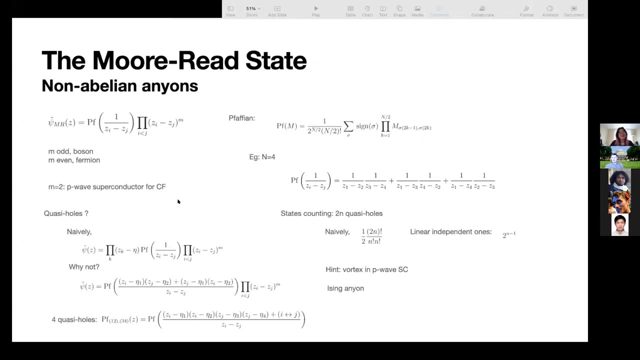 Thank you, Yeah, I. so I had one question. Sure sure, When you wrote down the Moore-Reed state, you said for m equals 2, it's a P wave superconductor. Yeah, yeah, And so I was wondering if there's. 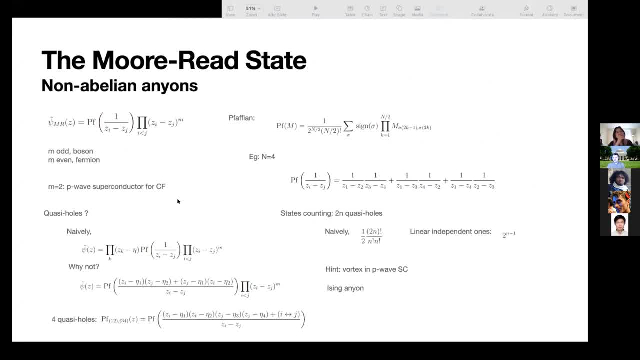 any physical way to understand this, like: is there some sort of instability to pairing, or is it just like we're writing down this state and it is the description of a P wave superconductor? Yeah, so the instability question really depends on the Hamiltonian right. 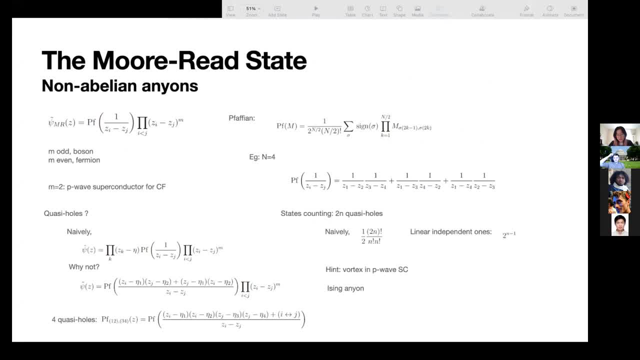 Right, So yeah, but here I just proposed some kind of. I just proposed a wave function for this state. I don't have any. yeah, it's not a statement of the instability. Got it OK, thank you. Yeah, I have a question. 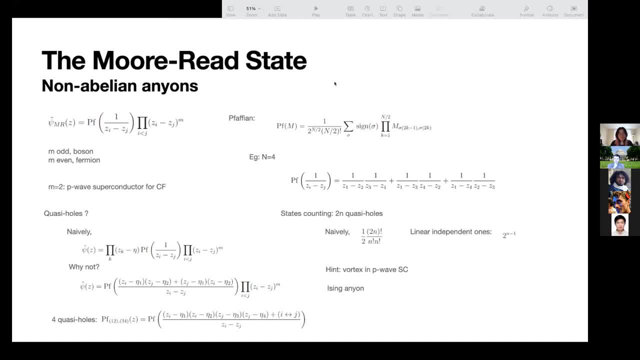 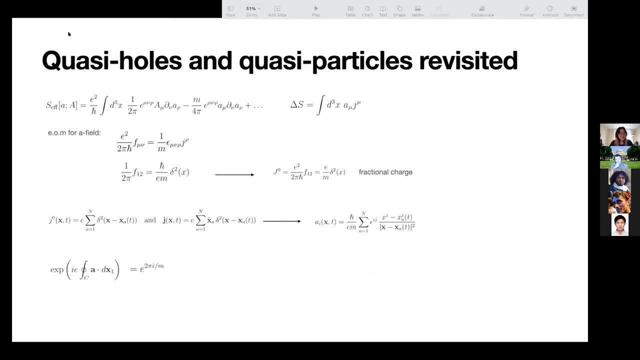 So you were talking about how the Chern-Simons term plus a Maxwell term leads to a gap for a gauge field, right? Yeah, Yeah, you said this is like what we want, sort of, But I don't know, it's kind of surprising, right. 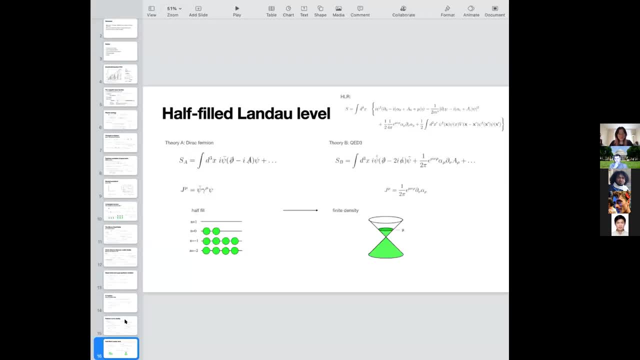 Like you, couple a gauge field to a bunch of gap stuff and then somehow that gap stuff manages to produce something, Yeah Yeah, It produces a gap in the gauge field itself too, right, So why did we expect the response theory to have a gap? 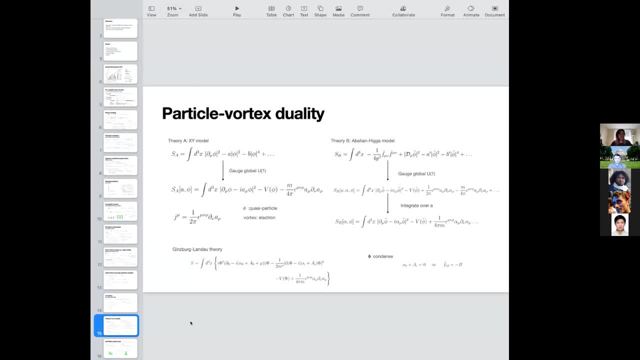 Oh, I mean, I said that, based on this, based on that, we want to get an effective field theory for quantum core states. right, So we want to gap, so we want it to be gapped. Well, so the matter, well, so the matter is gapped right. 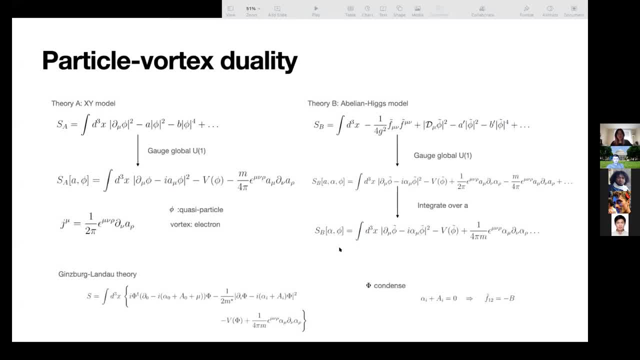 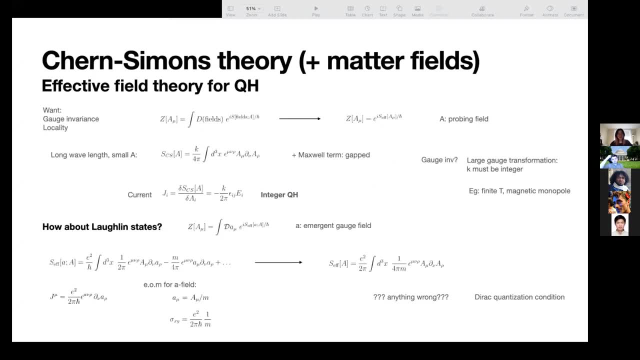 But so am I correct in imagining that capital A should be thought of as like the electromagnetic field minus the magnetic field that's causing the quantum Hall effect? Or is capital A something else? Yeah, yeah, yeah, right, right, OK, OK. 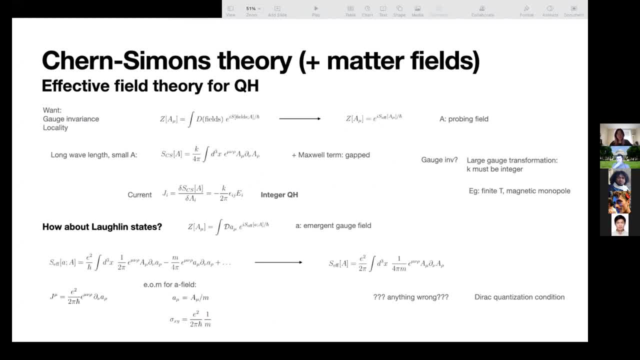 But like if I were to just couple a gauge field, if I were to just couple a to a massive field, right then coupling a to a. so if I had like for a plus a coupled to a massive thing, right then. a would definitely not be gapped. 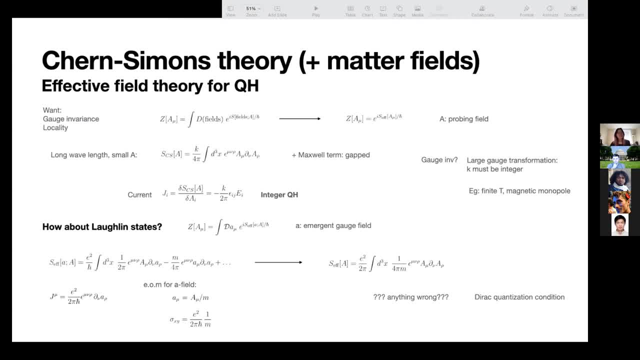 right, I would just ignore the coupling to the massive thing, right. And so here, if I don't add any a, I still have a bunch of gapped matter, right? But then the claim is that I can couple a to this gapped matter. 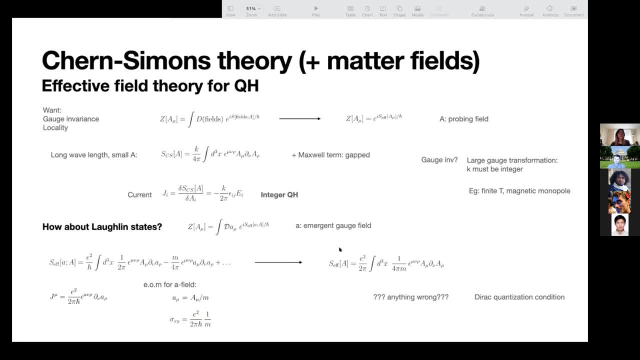 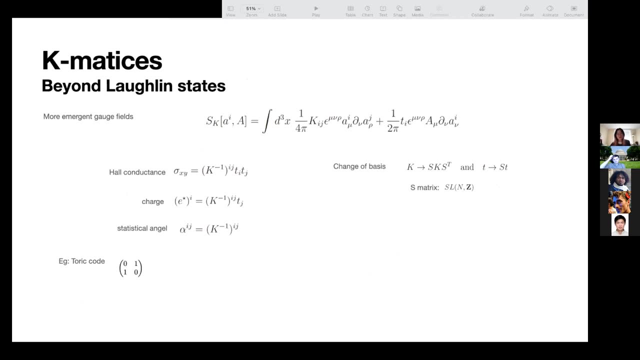 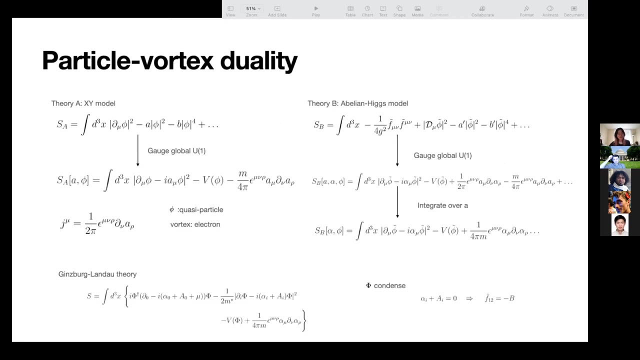 right, And then it'll produce this quantum Hall and then lead to a gap in the A, which is kind of interesting. Yeah, I mean, in this one way to think of it is in terms of this, in terms of the HRI. 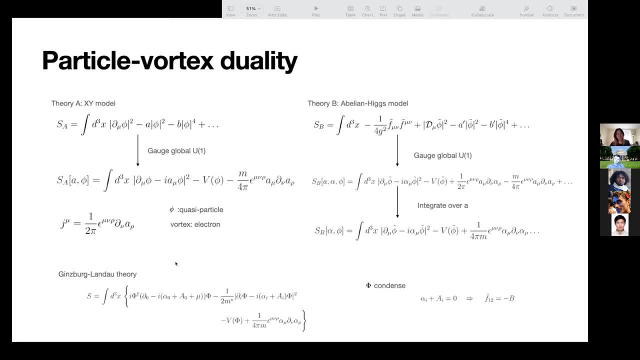 HRI, HRI theory, right. It's like, yeah, it's similar to something like this. So, Yeah, you have to. you want to be coupling a to like a Higgs field or something, right? But Yeah, yeah. 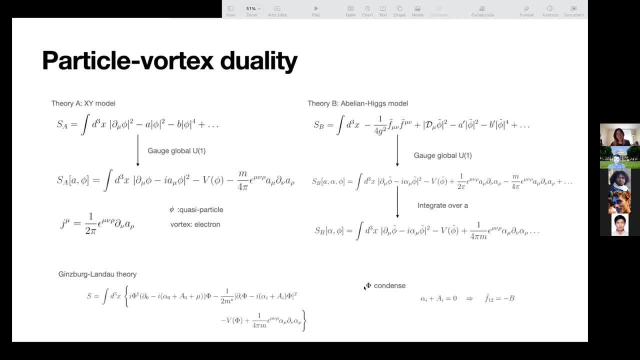 I guess that's pretty obvious, that this is the right. this is what's going on in quantum Hall, right? OK, maybe you're saying that using particle vortex duality is the best way to understand it. Yeah, I think that's one good stuff about you, know. 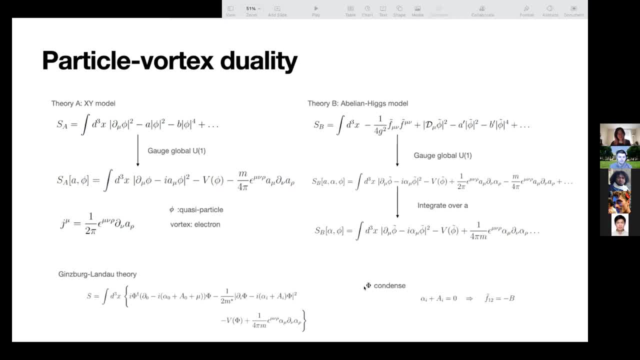 the stuff about particle vortex duality. OK, And then. so the other question is then: I mean, you're talking about the direct quantization condition being important. Yeah, yeah, Yeah. So, but if a is supposed to capital A, 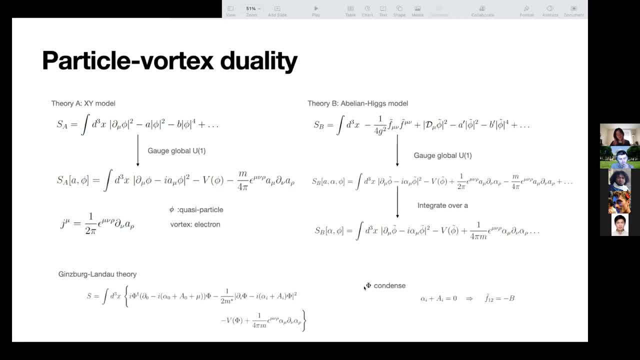 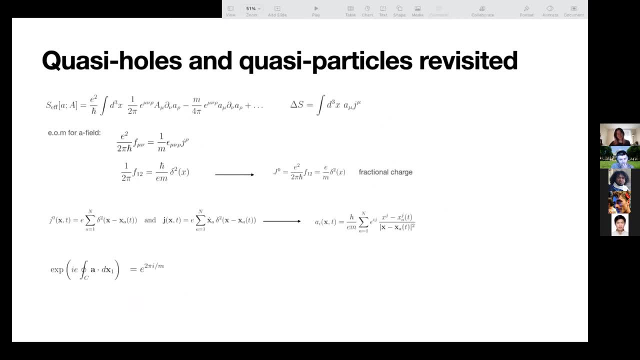 is supposed to be like the physical electromagnetic field minus the magnetic field part. then I mean in, like a real, in a, And maybe this is too pedantic, but in a real sample capital A should still have its quantization condition fixed. 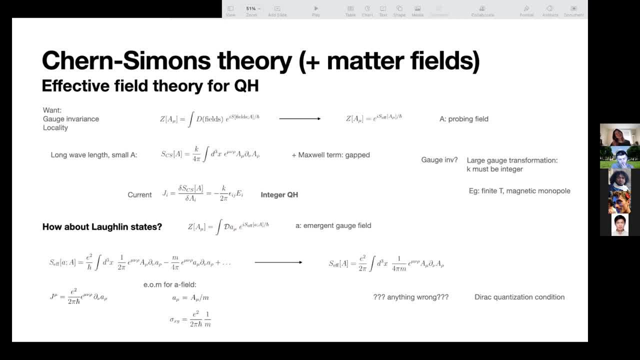 as in a normal charge 1 field, right? Yeah, Like if it's the physical electromagnetic field, right? So are we just saying that it's impossible to consider like a scenario where you only have one source, You only have like a 1-mth flux or something? 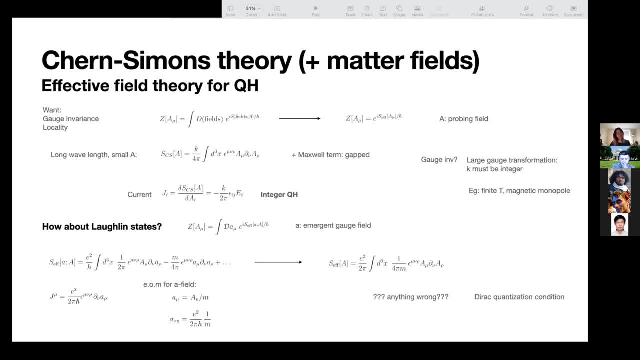 Because there are no field configurations where you can create a 1-mth charge in reality. So that's why it's OK you're saying so. And also, this equation of motion is equating the field strengths, not the gauge fields themselves. 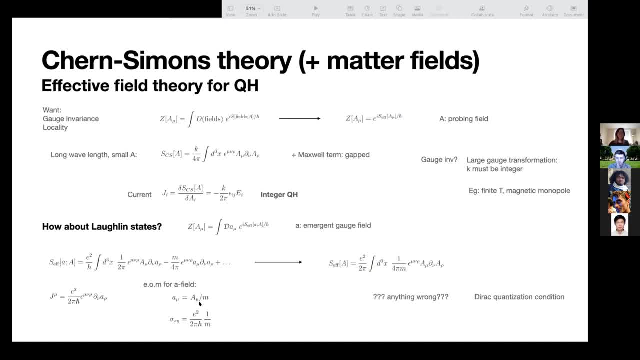 Yeah, yeah, yeah, So, So there should be plus something. Yeah, I didn't write it down. Yeah, yeah, this is an equation of field strengths, Right, so yeah, so back to the question. But, like, the field strength doesn't care about this holonomy. 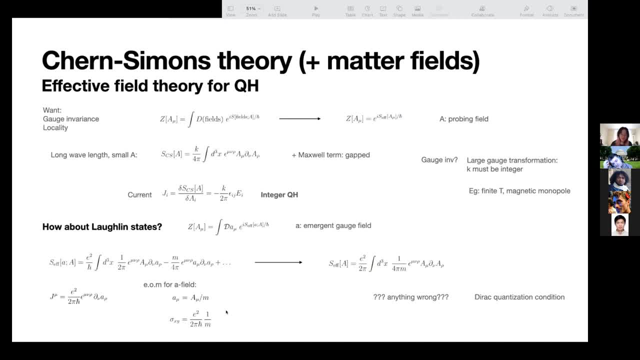 part right. If I just say the two field strengths have to be equal, then why do I say A Right? yeah, But at the end of the day you get something that's so. the field strength doesn't care about this. 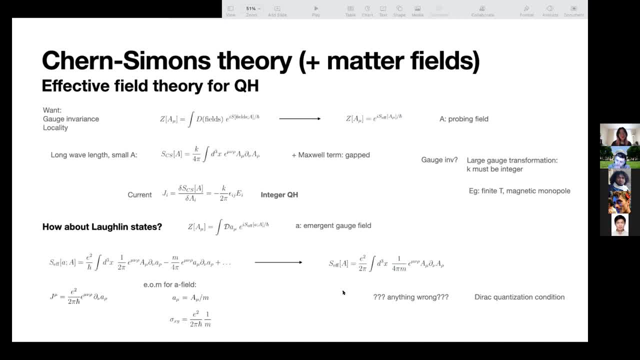 There are quantization, But at the end of the day, we want the effective action to. we want a gauge invariant theory, right? So I mean it seems that by putting a non-integer in front of the transcendence term, the theory might not be gauge invariant. 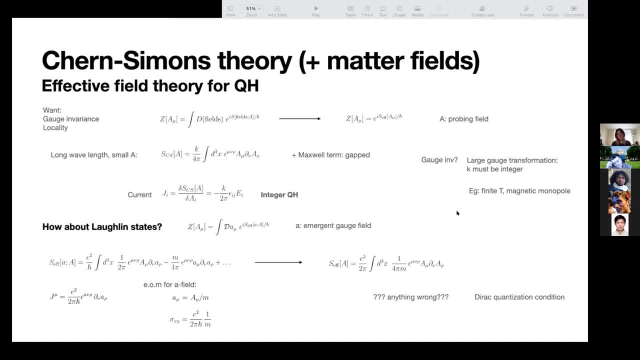 Well, yeah, and I would say that that's true, because the equation of motion you're using was not the real equation of motion. What do you mean If you're using the equation? I agree, you can use the equation of motion to set the field. 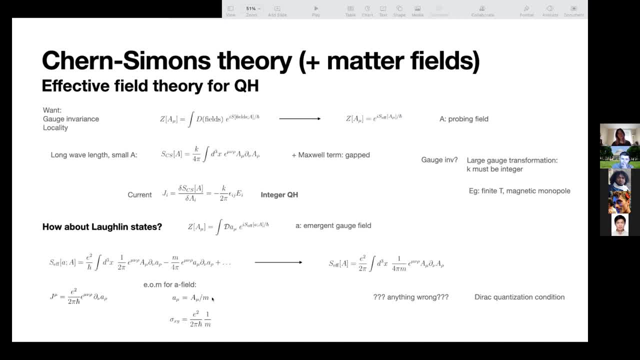 strengths equal to each other. right, But how do you know that It seems like you get- I mean, it seems naively, that you get- something that doesn't make sense if you also set the gauge fields to be related by its factor of 1. 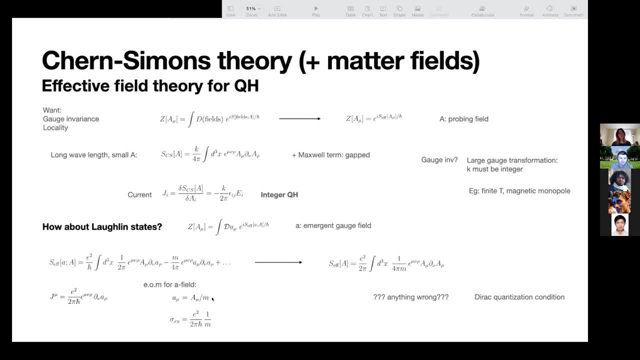 over m right, Yeah, yeah, Yeah, that's true. So I would have. I would have thought that we ran into a problem because we used- we pretended like the equation of motion was for the gauge fields instead of the field strengths, right. 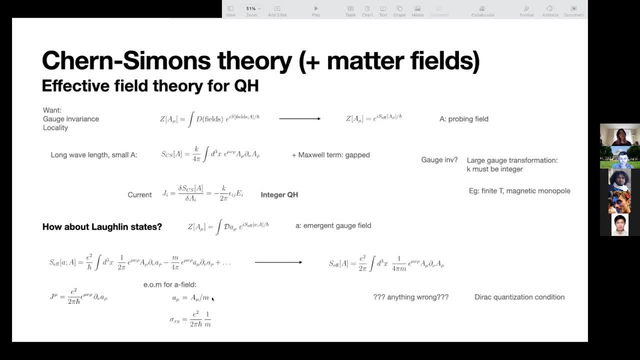 But then you're saying that there's actually no problem in that using setting the field strengths like this to be related in this way is actually makes sense, right? Yeah, it actually makes sense. I mean, locally, it doesn't care. 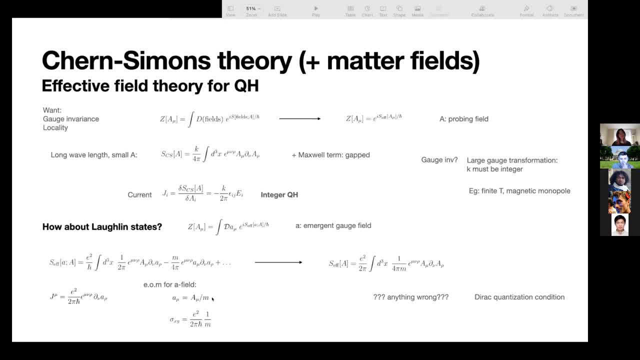 The field strength doesn't care about this monopole stuff. I mean. I mean, this is a legitimate equation But the. so the but the direct quantization for capital A should still should be the regular thing, right, The direct quantization for capital A. 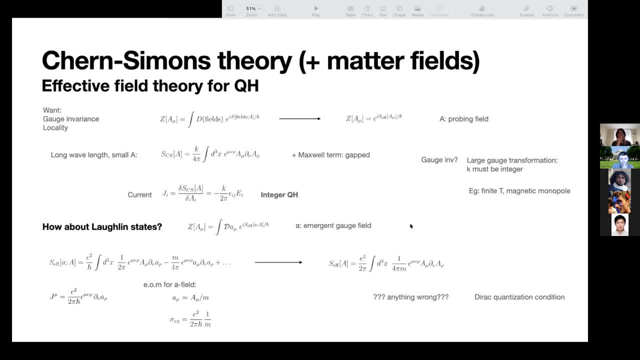 Right. So this is. this is effective with the 1 over m Would make sense if I can only consider magnetic fluxes of strength m for A right. Capital A, Yeah, right, Yeah. But capital A is the physical electromagnetic field. 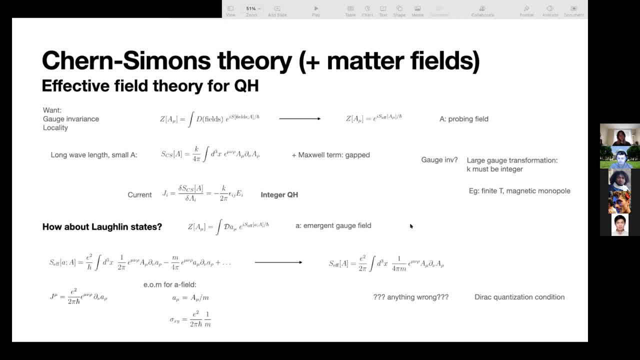 So I can definitely consider a 2 pi flux for capital A. right, Yeah, you can definitely consider a 2 pi flux for capital A, But yeah, But then don't, I doesn't. isn't there something, indeed something, wrong with that? 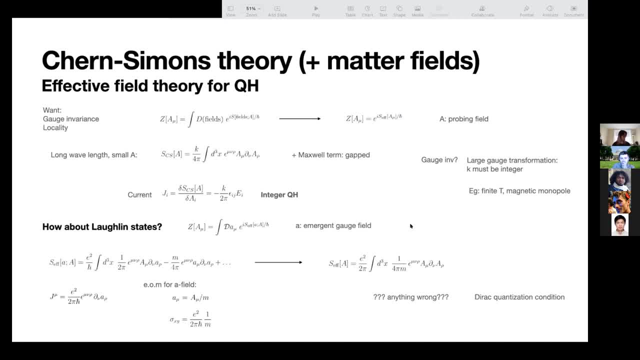 Yeah, I would let me do one more test, Because it's a 3-point microscope for recall, with the 3 to m point mushroom. So this is the basic story and this is the. this is, you know, it's a good example. 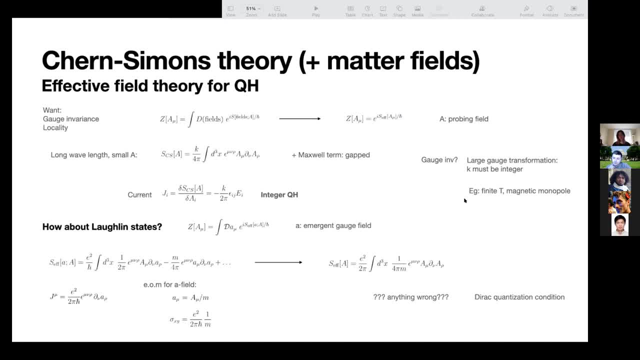 I mean by the original one, because the fundamental electric charge is always E. It's not E over M, Right, Right. But here we're actually considering a quasi-particle in this system. By quasi-particle I mean we can have M. If we inject an electron to the system, it will just split to M quasi-particles. 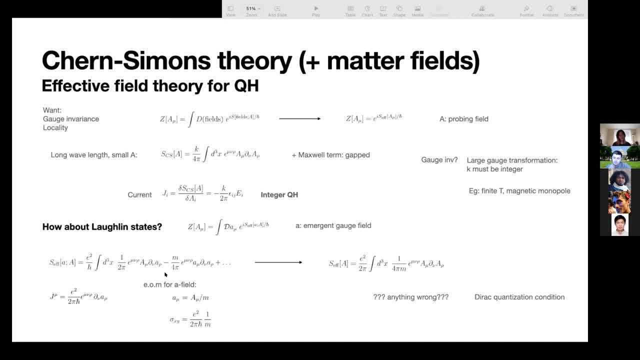 and then they can move arbitrarily far from each other. Yeah, So can I just say that this is equivalent to just pretending like I can consider configurations where there's only one quasi-particle. Yeah, Yeah, Even though that's not gauged invariant under the little a. 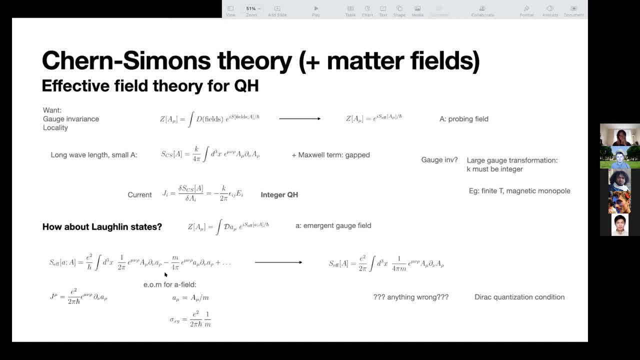 That's gauged invariant under little a. That will cause this term to be M, To be not gauged invariant. Okay, Maybe I'll just ponder this for a bit. Thanks, Cool. Any last questions? No, No. 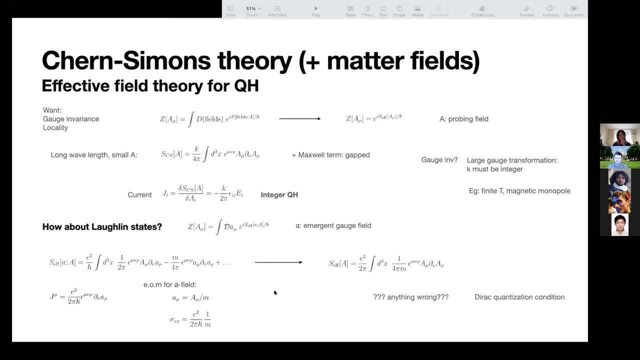 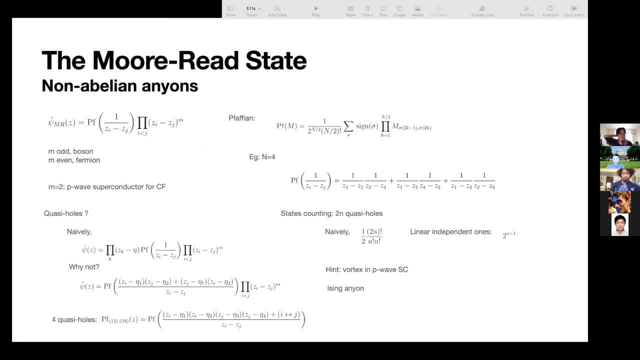 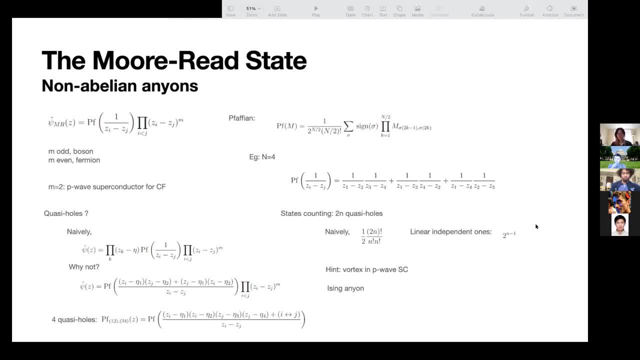 I've produced this Fafion. So is there some physical understanding for this as coming from this Fafion, as coming from the Majorana fermions? in this way, I think by physical understanding, maybe you can think of it in terms of composite fermion. 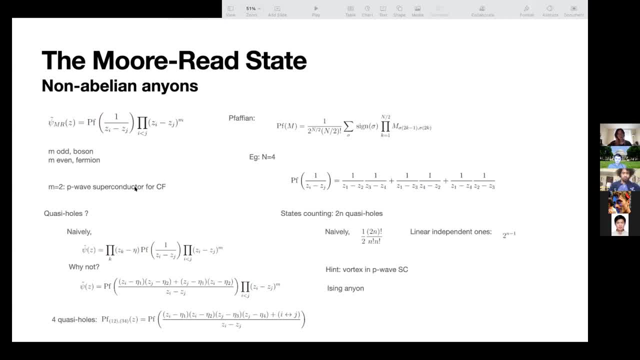 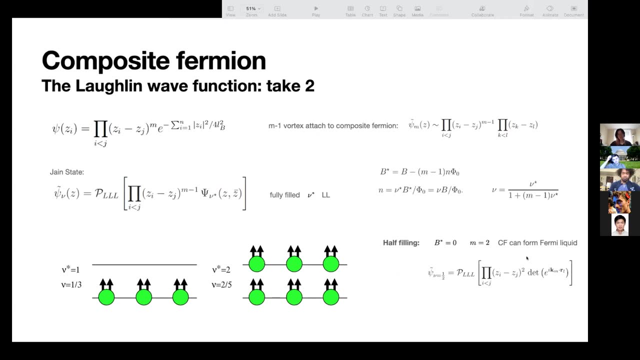 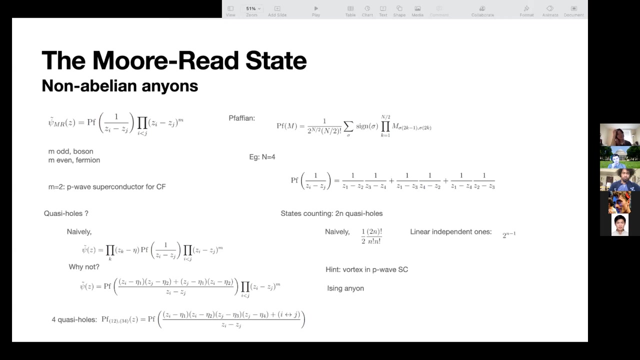 Yeah, I mean in terms of composite fermion. this is a p-wave superconductor for this composite fermion And I think you can- You can get this by starting from the composite fermion. fermi liquid, Oh OK.